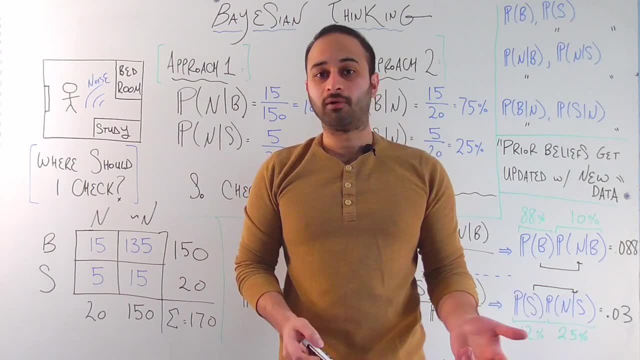 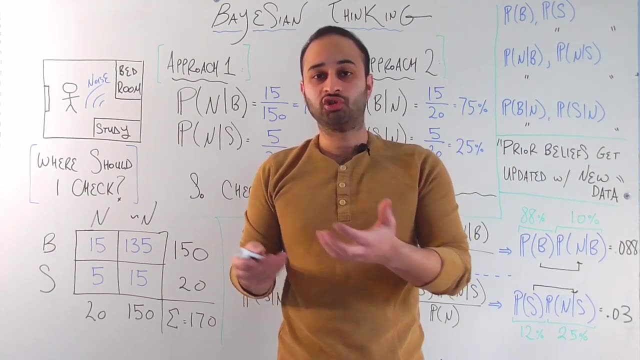 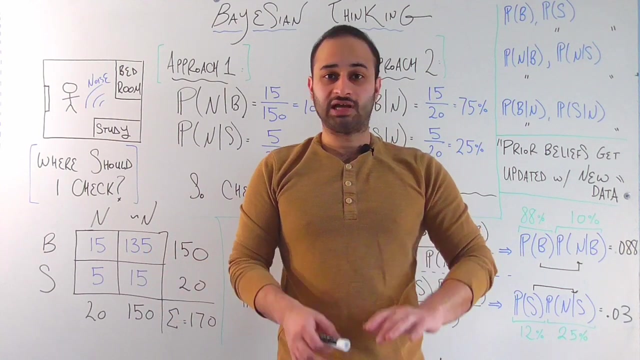 would either one be better? What are the pros and cons of each one? So in this video I purely just want to explain to you the pros of thinking in a Bayesian way and also some of the cons. We're not going to be going over any like high-level stats at all. We're going to be using a very down-to-earth 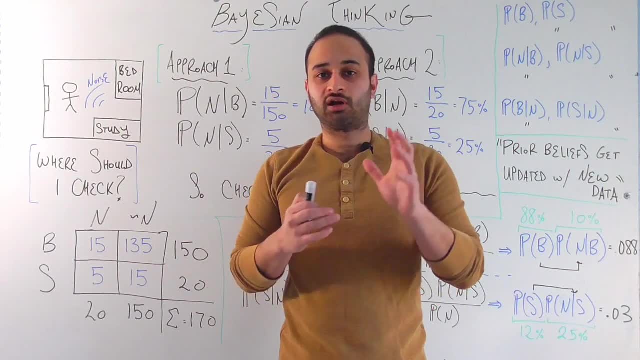 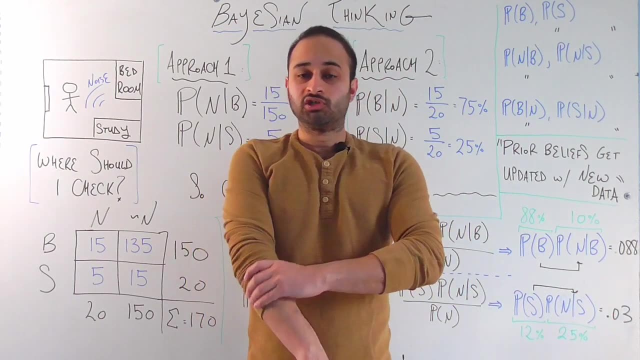 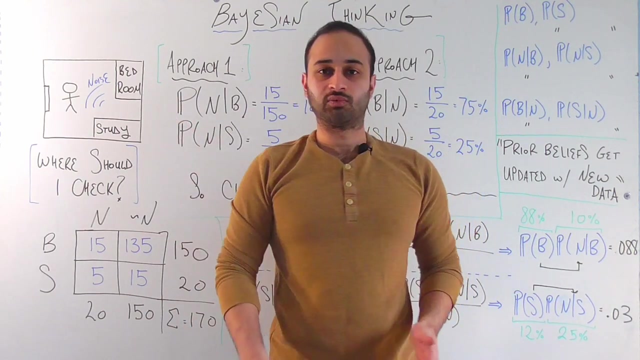 problem and hopefully, using this example, we can kind of start understanding why it would help to think in that way, or what are the costs that we pay to think that way. So here's the example. So let's say that you live in an apartment and this apartment just has a bedroom and it has a study. 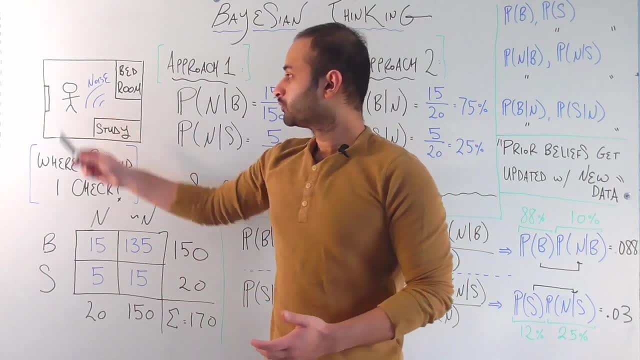 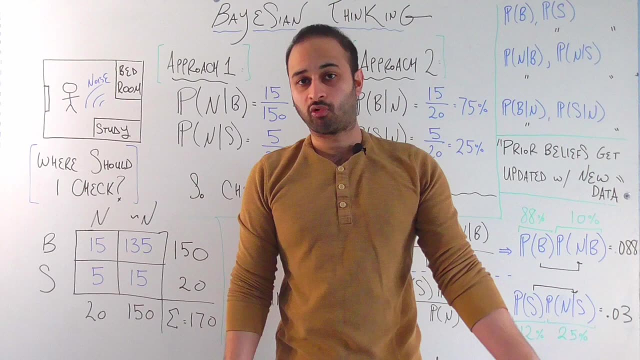 So we have two rooms in the apartment and this is you, and the problem that you face is that you are always forgetting your cell phone in one of the two rooms before you leave for work in the morning. So you either have left your cell phone in the bedroom or you have left it in the study, So you always 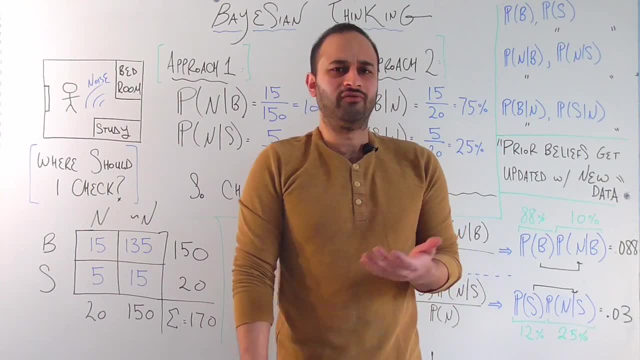 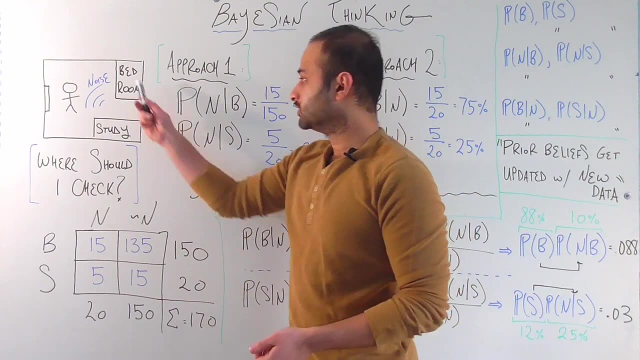 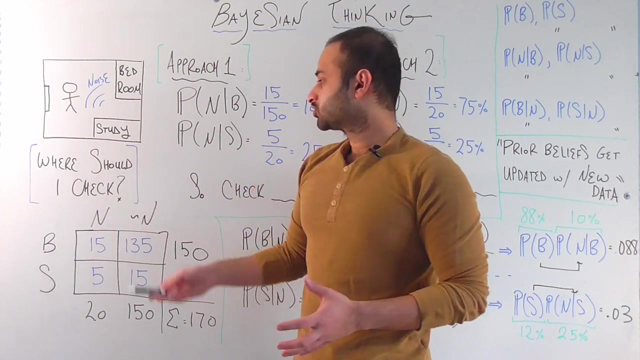 have to go back into your house. You use your landline- and who even has those anymore? but you have a call, your cell phone It starts ringing and you hear a noise from somewhere. That noise is either coming from the bedroom or the study, but you can't precisely pinpoint it and the natural question is: where should 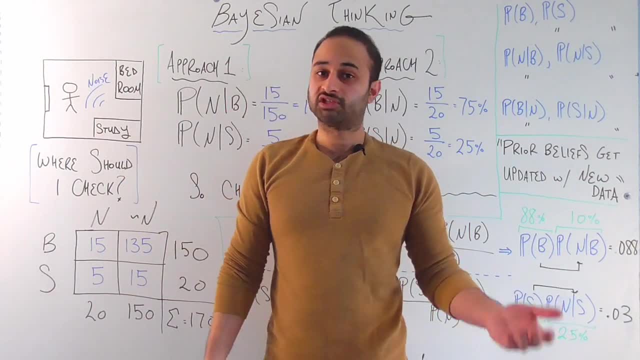 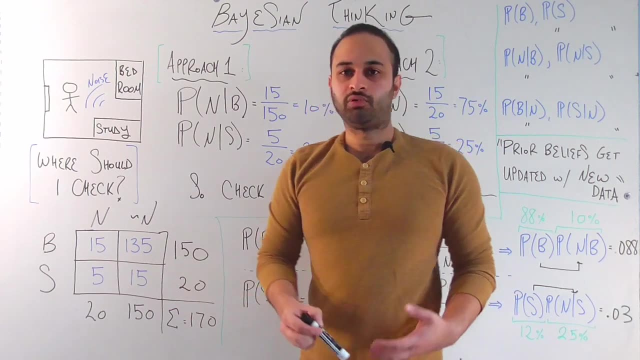 I go check. Should I go to the bedroom to check for my phone, or should I go to the study? Now let's bring in a little bit of data to help us make our decision. So here's the data we'll be using for this problem. 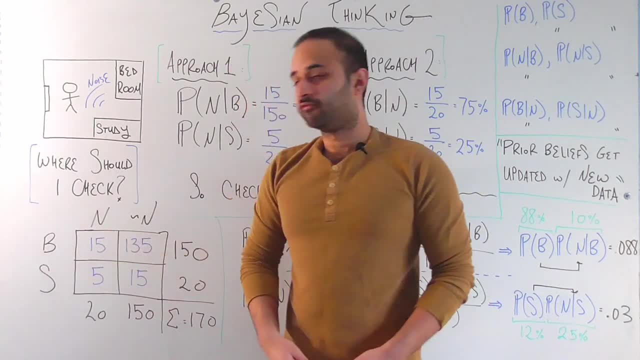 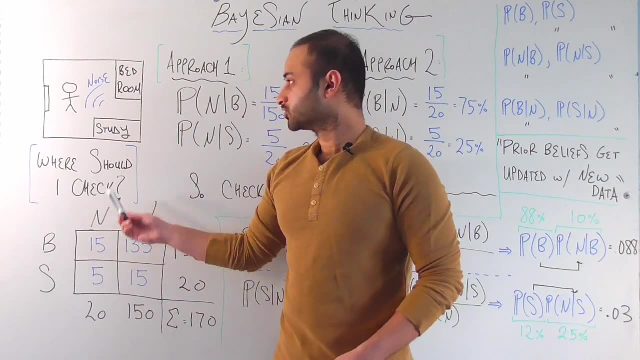 Pretty simple, two by two table. The rows are whether the phone is actually in the bedroom or the study. So B is bedroom and S is study, And the columns are N, which is the noise. So the columns are whether you hear the noise or you do not hear this specific noise. 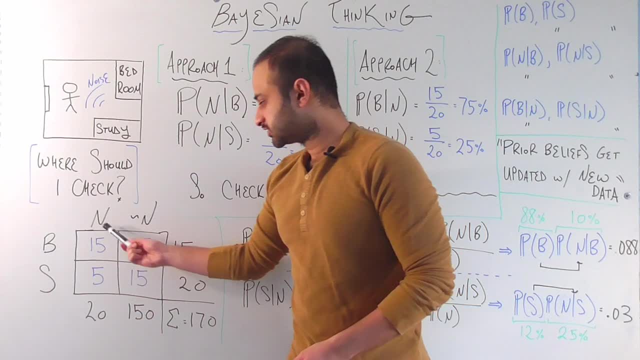 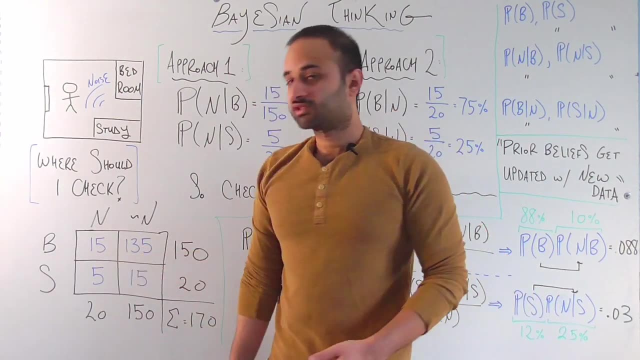 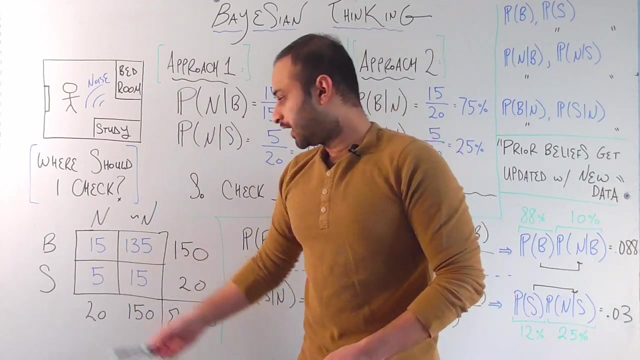 You hear a different noise, So how to interpret this table? for example, what does this 15 mean? This means that of all the times you've lost your phone in the past year, 15 times you have heard the specific noise that you're hearing right now, and it's been in the bedroom Five times. you've 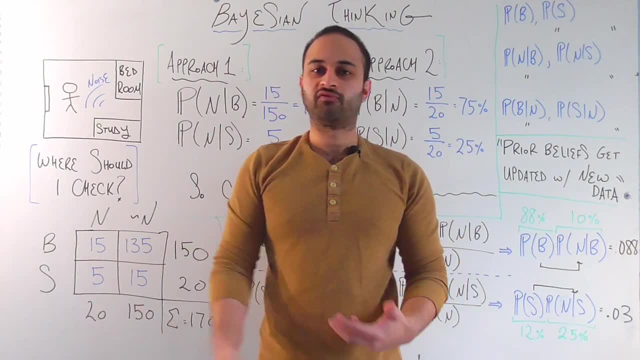 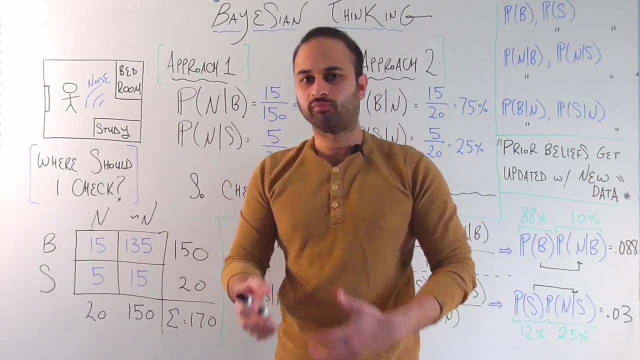 heard the specific noise that you're hearing right now, but it was actually in the study and the reason for this uncertainty is, you know, your apartment has like echo to it. you might not hear things one day and you might hear things another day. so there's some variation, some randomness. 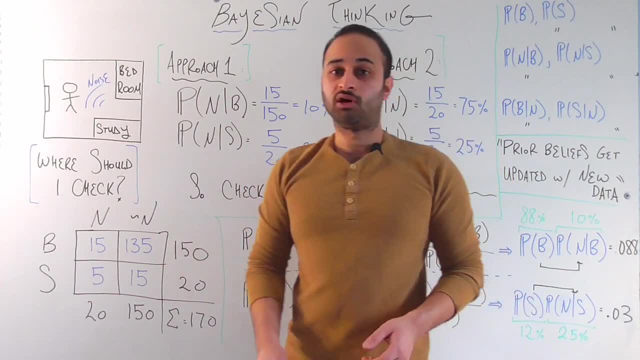 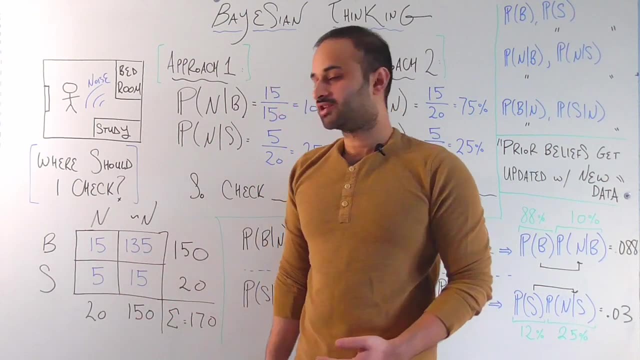 built into this problem. 135 times you heard some other noise, so tilde N means not this current noise. you heard some other noise and it was actually in the bedroom, and 15 times you heard some other noise and it was in the study. So how do we use these four numbers? How do we use this data in? 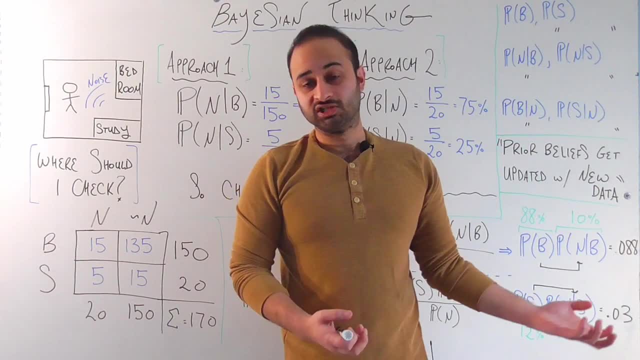 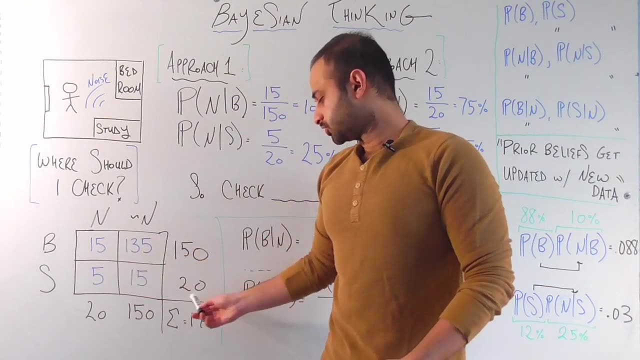 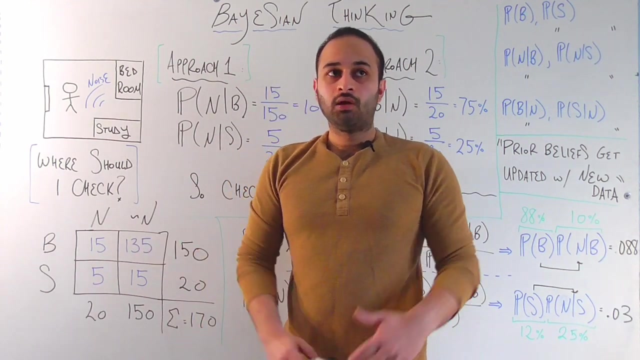 order to make some kind of well-founded decision about where are we going to be able to find the noise. This is where I should go check and, by the way, the column sums are here, the row sums are here, so there's a total of 170 observations, or days worth, of your phone being missing in the data. 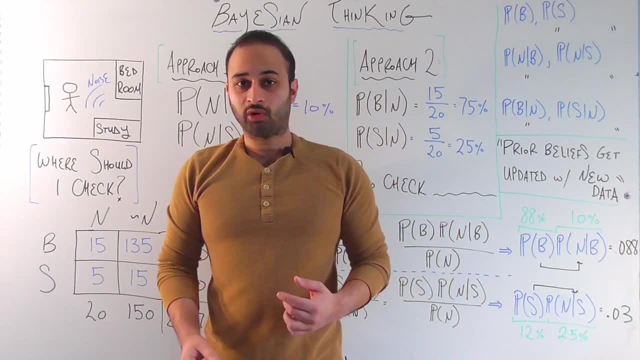 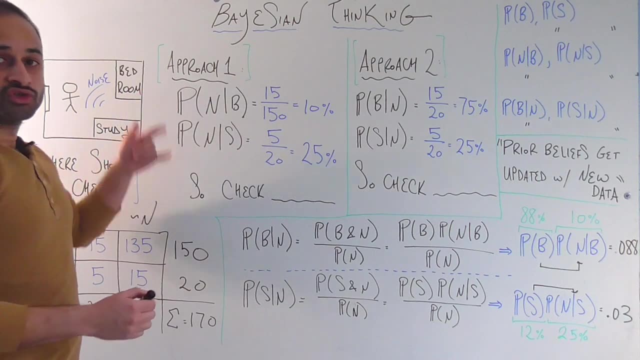 Let's do. approach number one- and this is the non-Bayesian way- and we're going to do this so that we can kind of go from there. So approach number one says that I'm going to calculate these two probabilities, these two conditional probabilities. The first one is the probability that you hear. 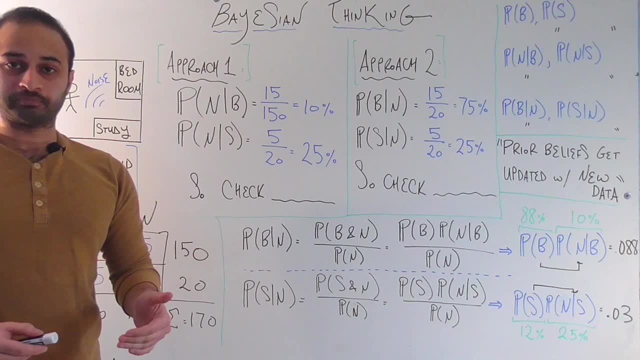 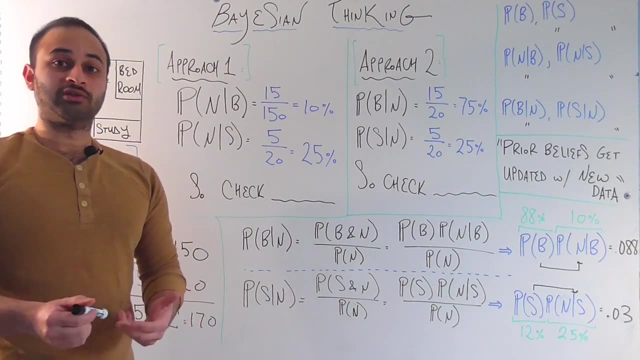 this noise, given that your phone is actually in the bedroom. so again, intuitively, this is saying that if my phone was actually in the bedroom, what are the chances that I would be hearing this noise right now? and we can compute this by looking at the first row. so this is all the cases where my 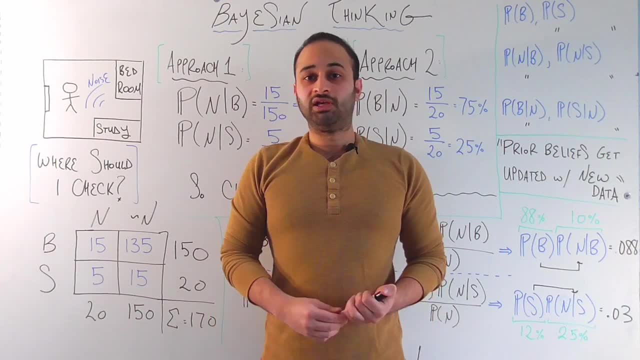 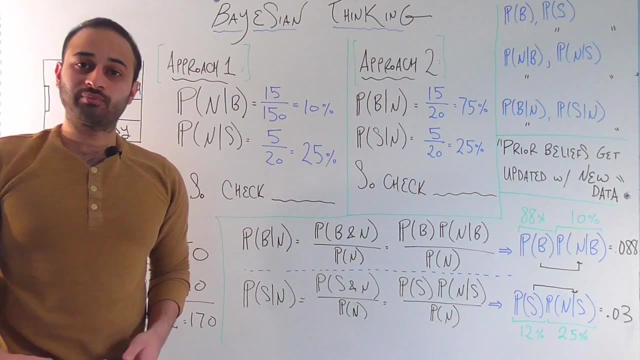 phone is actually in the bedroom and the probability I'd be hearing this noise is 15 cases out of those 150, which is 10 percent. So there's a 10 percent chance that if my phone was actually in the bedroom, I would be hearing this noise right now. Similarly, you can check. 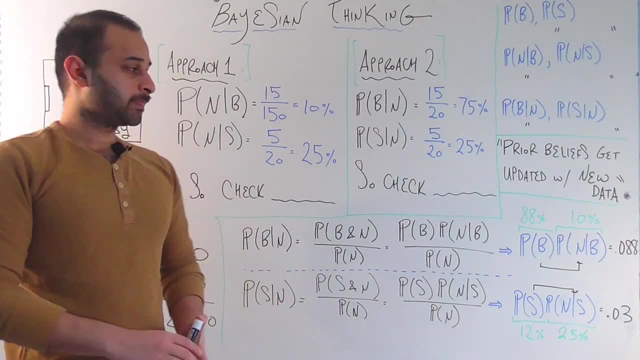 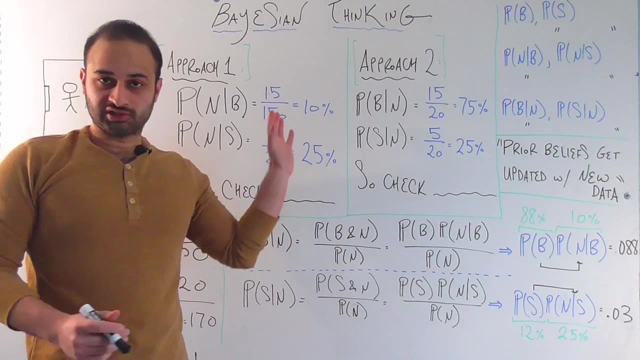 for yourself that if the phone was actually in the study, the probability that I'd be hearing this noise right now is 25%, And so, based on this data, I ask you, looking at just these two numbers alone right now, where would you go check? 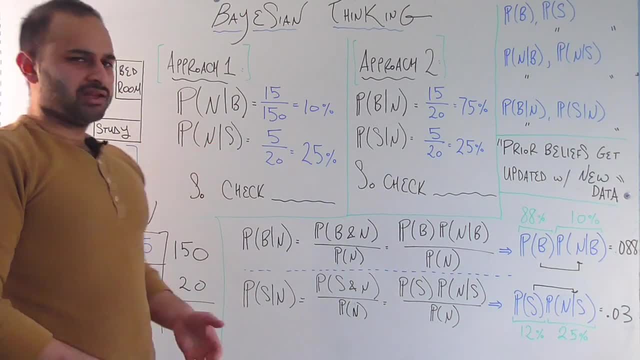 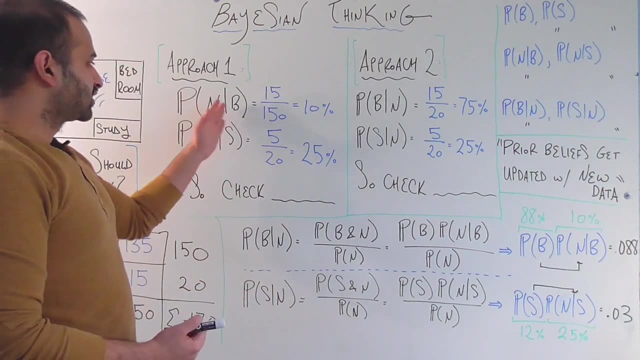 for the phone And I think most people would say I would go check the study And let's kind of elaborate on that a little bit more to build up this idea of why. why are we saying this conclusion? So if we look at this conditional probability, 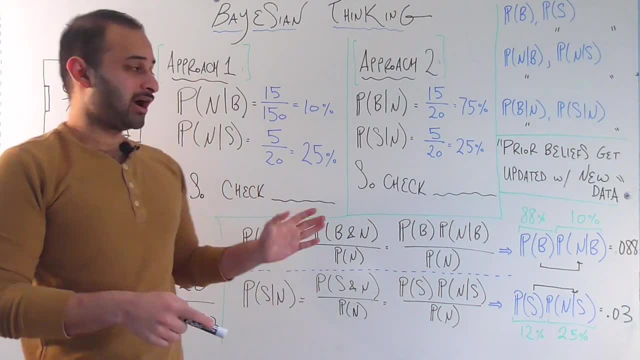 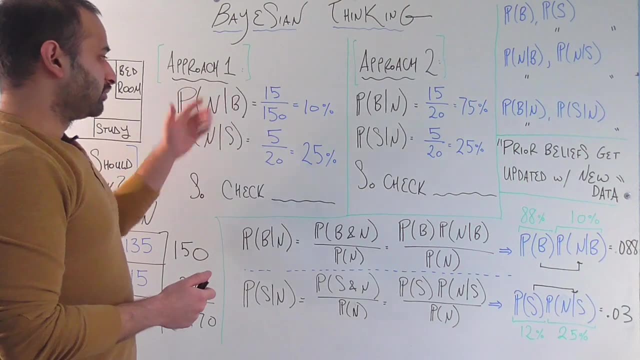 one of these things is known. one of these things is unknown. The right-hand side is unknown, because that's saying: where is my phone? Of course I don't know that for sure, but I know that if my phone was in the bedroom, then the thing. 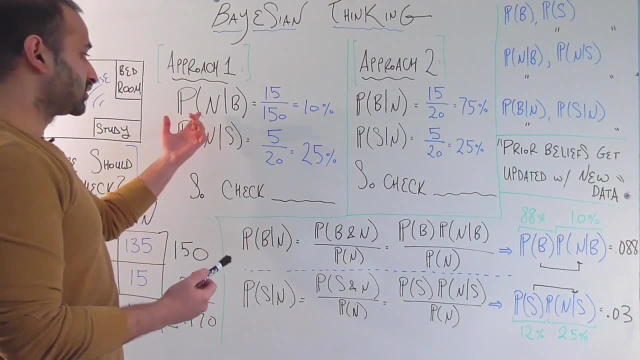 that is known, the thing that I am actually literally observing, which is the noise, would have a 10% chance. But if my phone was in the study, which is again unknown- then the chances of hearing the actual thing I am literally hearing are. 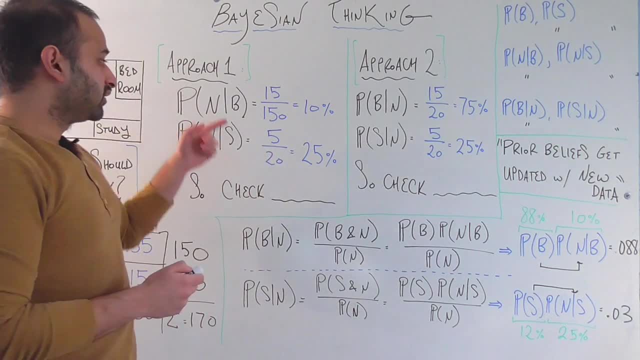 25%, And the natural conclusion comes from saying that, even though I don't know where my phone is, I don't know where my phone is. I don't know where my phone is. I know that one of these possibilities leads to a higher chance. 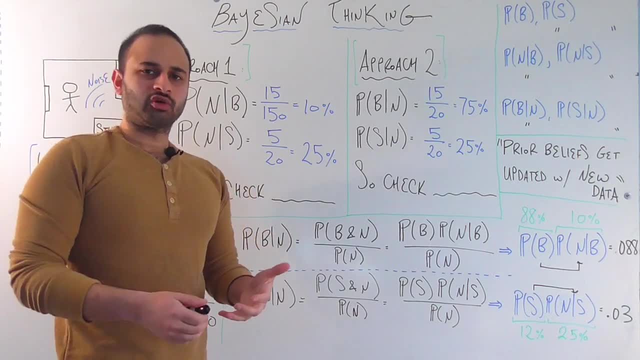 of hearing what I am actually hearing, And that's a very natural way to think about things. If you've studied some stats before, you know what I'm talking about is the maximum likelihood problem. We'll talk about it at the end of the 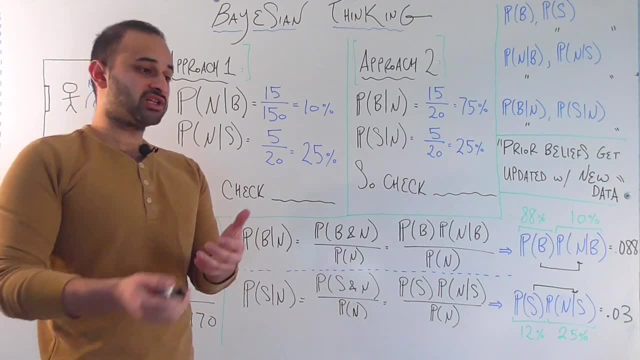 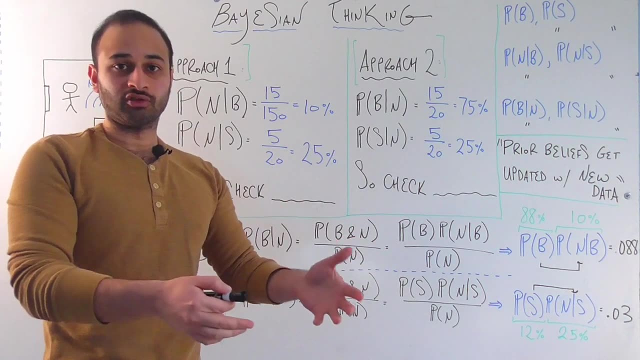 video, but before even assigning a name to it. this is basically saying that there is an event that happened in the world. What is the most likely state of this unknown quantity that would produce that event in the world? Okay, so if that's? 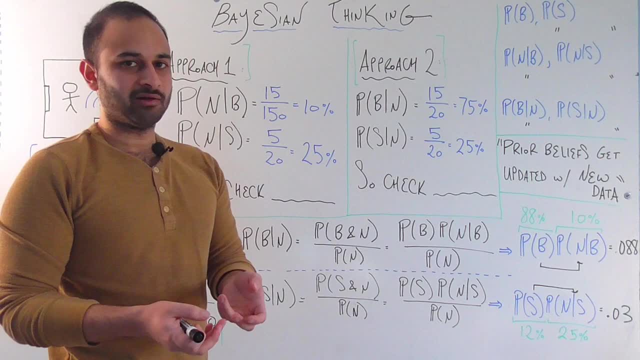 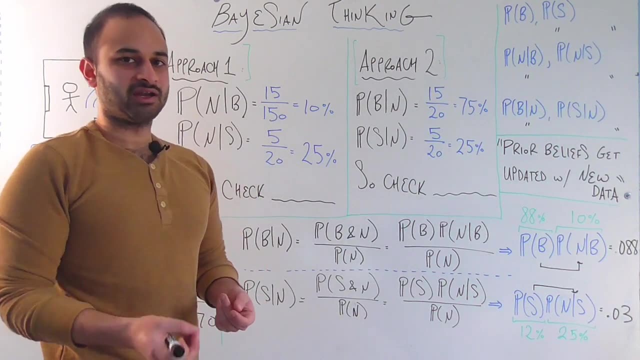 a little fuzzy, take a second to think about it. but we're just saying that there's some unknown event, but that unknown event generated some known data or known event, which is noise. What is the most likely scenario for that unknown quantity? And looking at this alone, we would say that it is in the 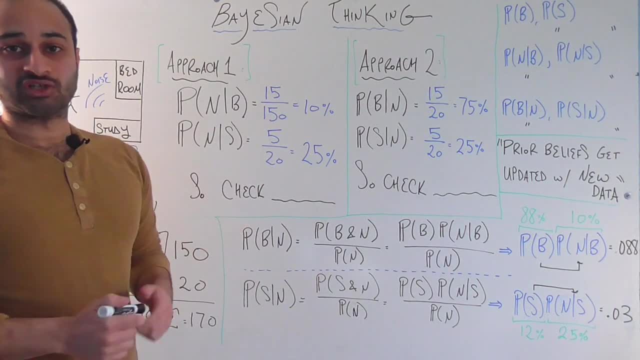 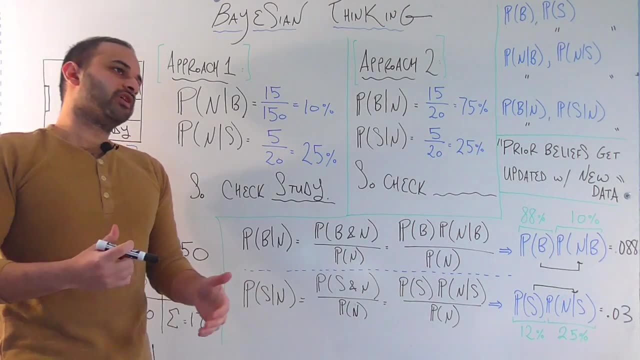 study, because that has a 25% chance versus a 10% chance. So, using approach number one, we go check the study and see if the phone is in there. Okay, seems pretty sound. Now let's think about this in a different way. And at first it seems. 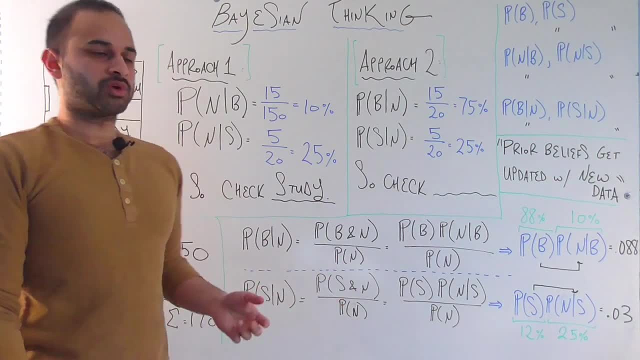 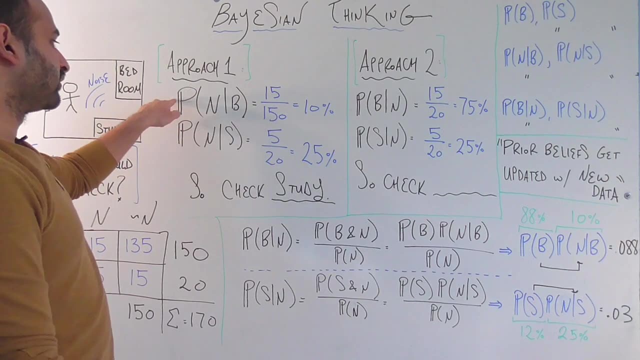 like I'm not doing anything crazy. Maybe we should get the same conclusion, because what I'm doing is just taking these two probabilities, these two conditional probabilities, and reversing their order. So notice, here I had probability of the noise given bedroom. Here I'm trying to get the probability. 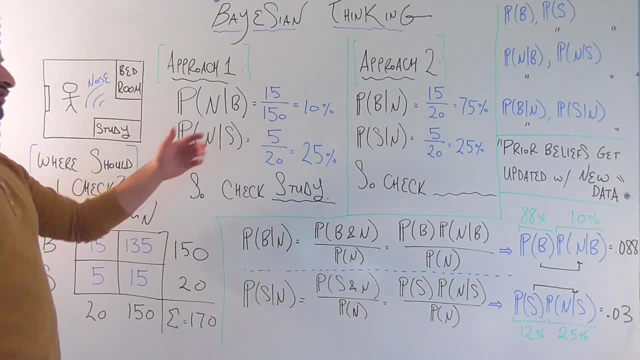 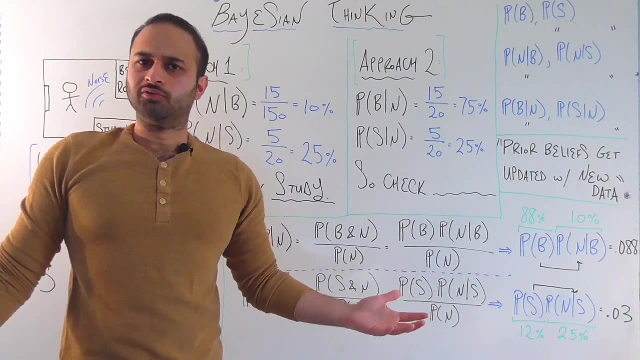 of the bedroom, given the noise. Here I had probability of noise, given it's in the study. Here I'm just trying to get the reverse- the probability that it's in the study, given that I hear the noise. So am I really doing anything different? 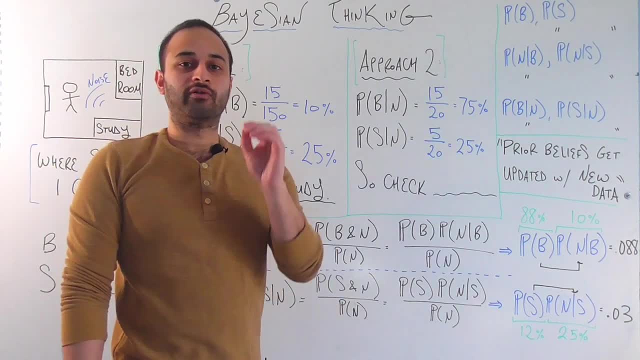 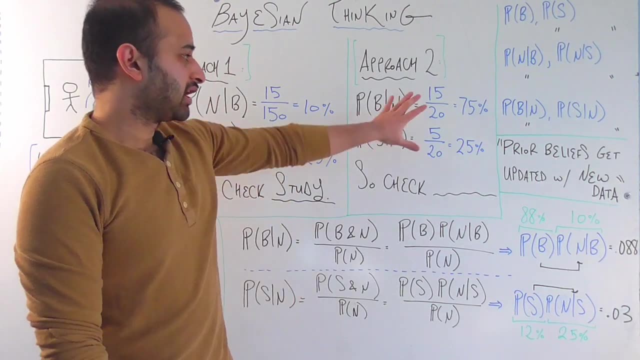 Well, it turns out I am doing something rather different, and we will go over the crux of this difference in just a moment. But first let's calculate the exact numbers and see what conclusion we get here. So, before I calculate the numbers, this is saying that what's the probability that my phone is in the 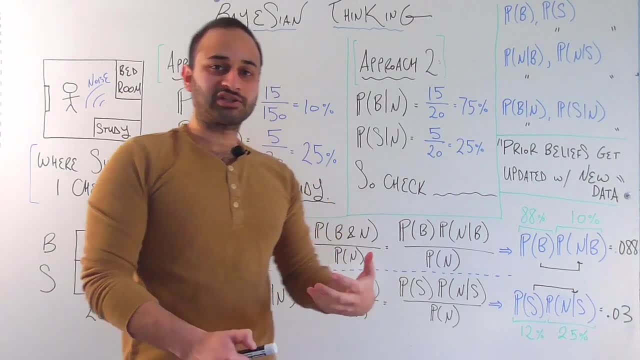 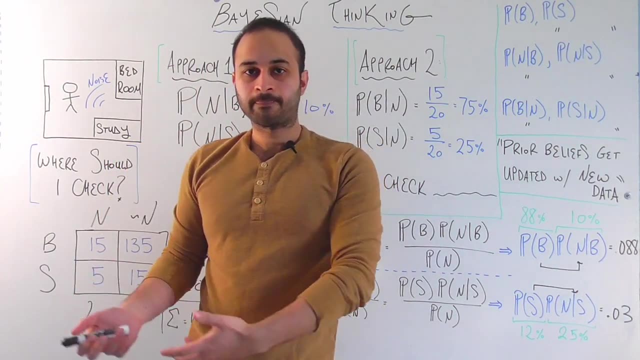 bedroom, given that I hear this noise. So this is asking a slightly different question. This is asking that, given that I heard this noise, given this observed data that I have just gotten, given that what's the probability that my phone is in the bedroom versus what's the probability that my phone is in the 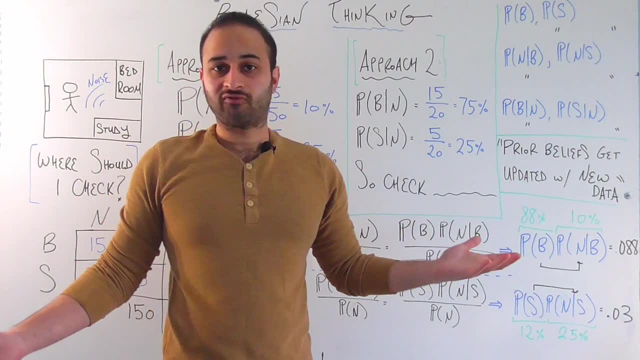 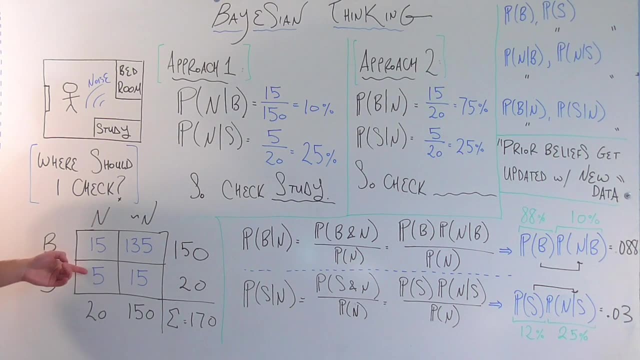 study. Now this quantity easy to compute again from our table. we just look at the column, which is n, so 15 times it's in the bedroom and 5 times it's in the study, and the total times is 20.. So that's why I have 15 numerator here: 5. 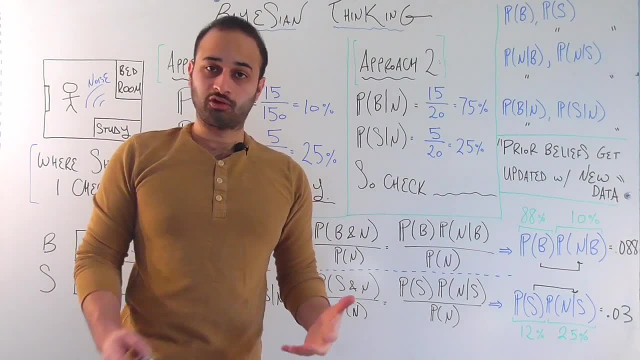 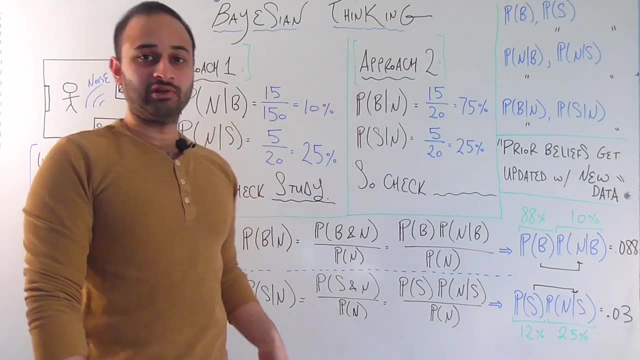 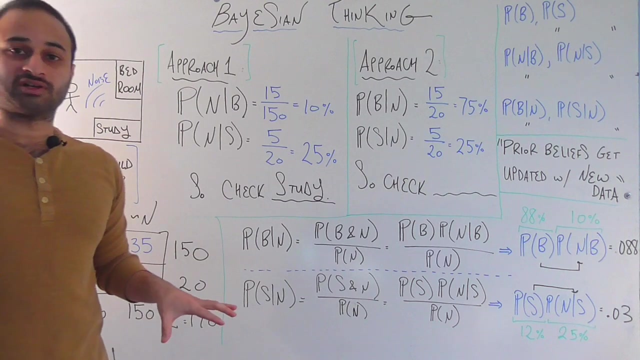 numerator here and these are my probabilities. Notice one quick thing: these two need to add up to 100% because I'm conditioning on the same thing and looking at all the possibilities for the item in the front. So these need to add up to 100%. but these probabilities don't need to add up to 100% because I'm 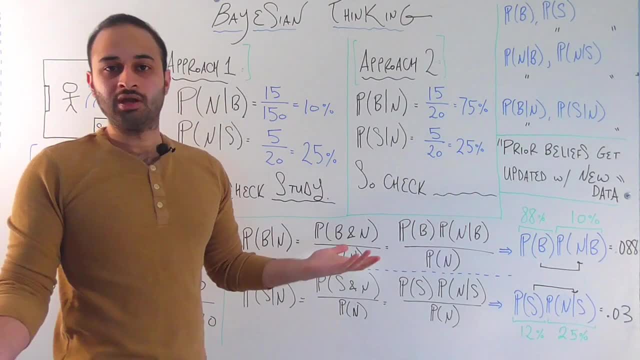 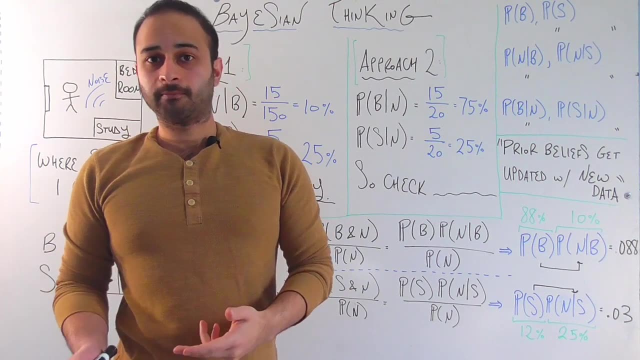 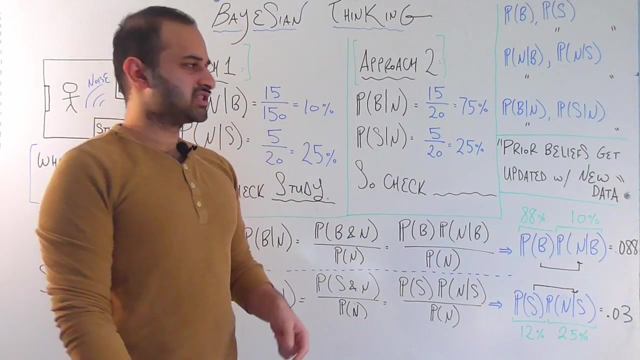 conditioning on different things, so there's no reason for them to necessarily add up to 100, okay, But looking at this data alone, where would you go check? It seems kind of paradoxical, because now it seems like I should go check the bedroom, right, Because what this is saying is that if I 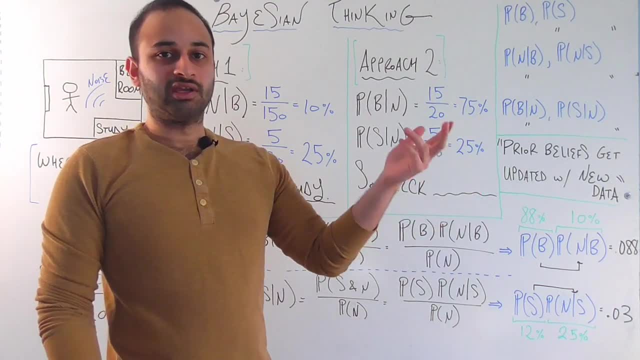 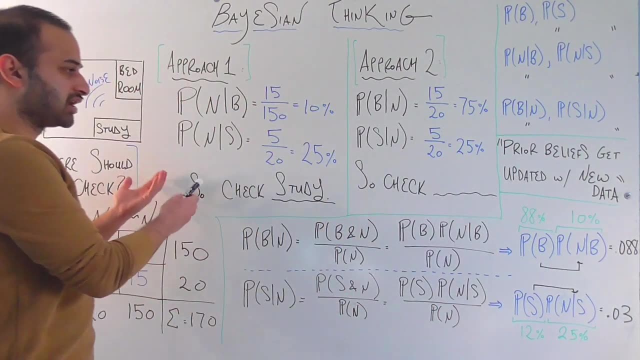 hear that noise, so that's a given. I've heard the noise. given that I heard the noise, what is the most likely place for my phone to be? That also seems like a natural question, just like this other one was a natural question. 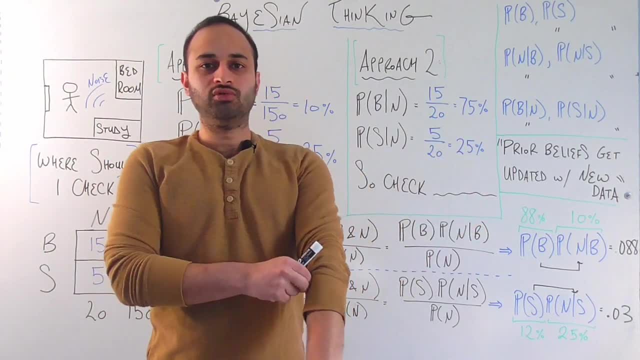 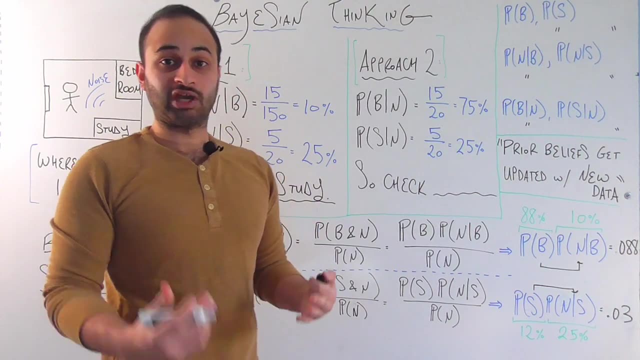 But even though they're both natural questions, they lead to two different conclusions. This one says that there's a 75% chance that my phone is in the bedroom. therefore I should check the bedroom. So on one hand it seems like: how can this be? How can I just flip the order of these conditional probabilities? 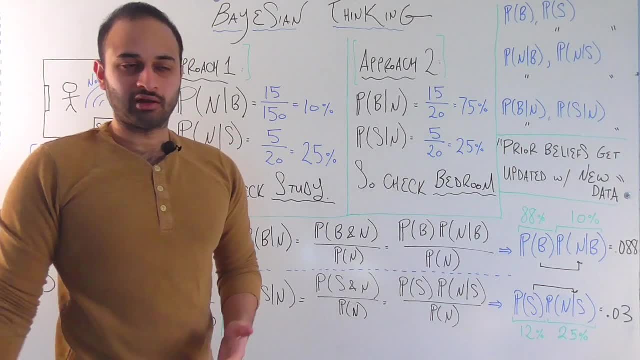 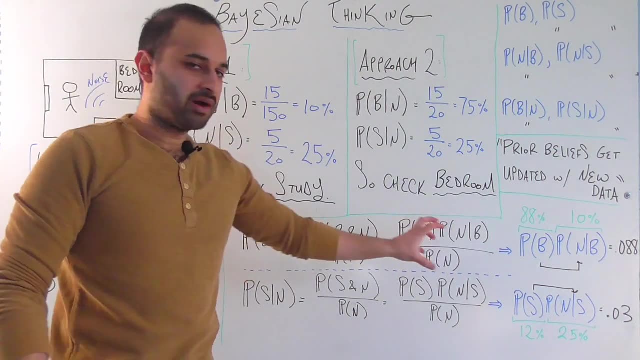 and I get a completely different result. To kind of understand that and understand why this is not a paradox in any way, let's take these two quantities and kind of break them up into their parts and see how the second approach that we're doing is actually very intimately related to the first. 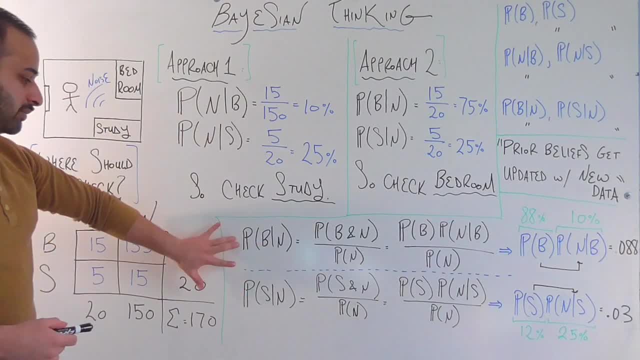 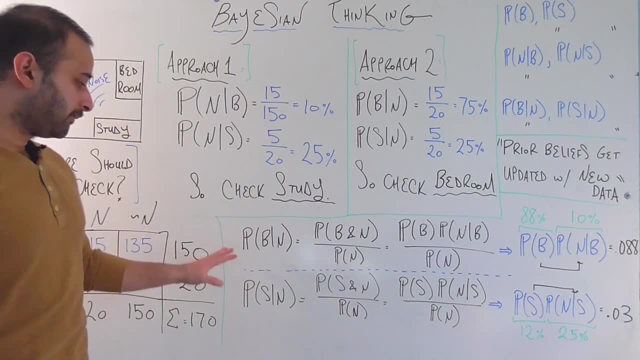 approach that we were doing. So that's what I'm doing down here. So I'm saying that these are my two probabilities again. So these two, same as these two. Now let's just look at how we can split up this probability here. The probability. 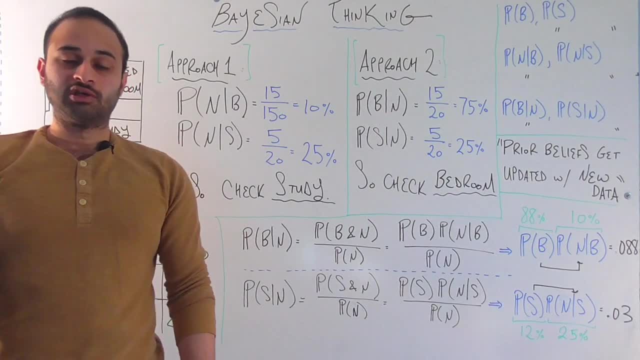 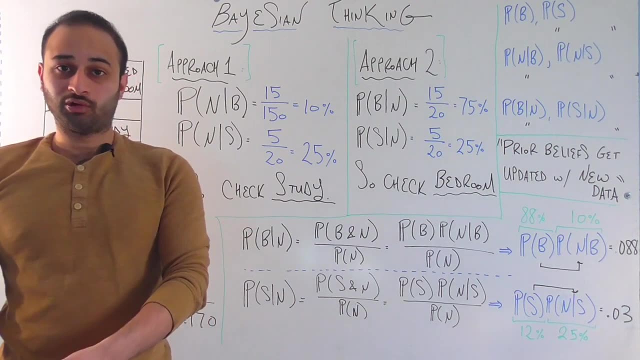 that my phone is in the bedroom, given that I hear the noise. so this is just going back to your probability 101, course, but this is equal to the probability of my phone being in the bedroom and I hear the noise, divided by the probability that I hear the noise. 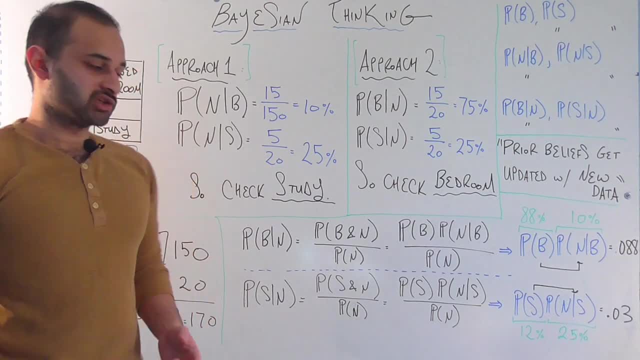 So this follows from, literally, the definition of what a conditional probability is. So I put the thing that's after the bar in the denominator, because I'm saying that, out of all these outcomes, what's the probability that I also have this outcome? So, definition of conditional probability. Now we'll leave. 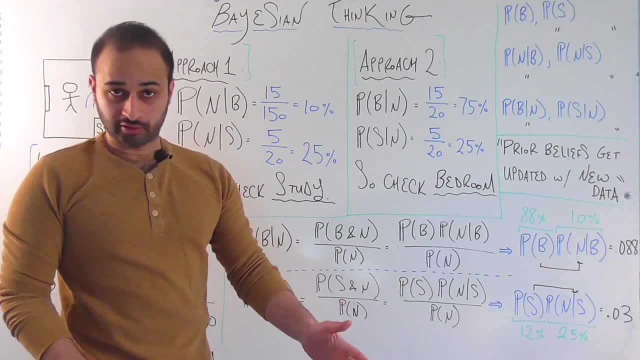 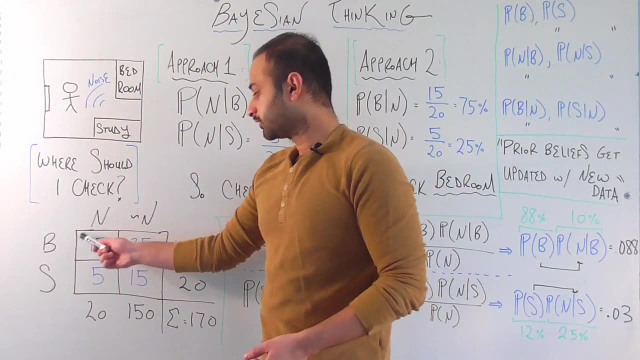 the denominator as it is, but let's process the numerator just one step further. So we're asking: what's the probability that my phone is in the bedroom and I hear the noise? So that's going to be this cell here. 15, divided by the total number of observations. 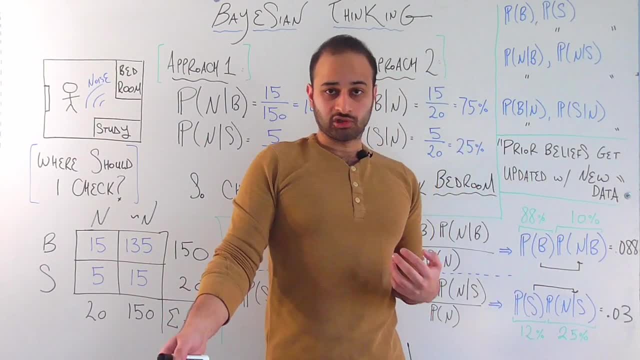 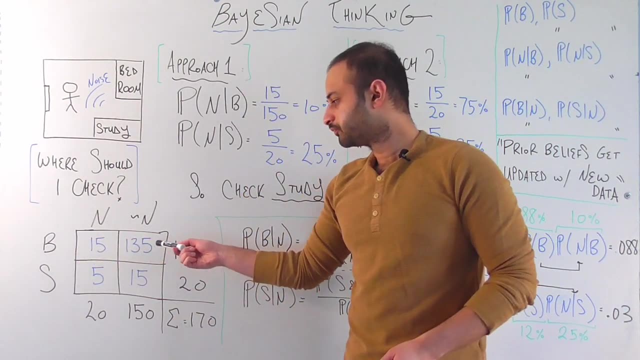 which is 170.. Now, a different way to get at that same result, that same probability, would be to do it in a two-step fashion. I could first say: what's the probability that my phone is in the bedroom? and then I could say, given that event, what's the probability that I hear the noise? That's exactly. 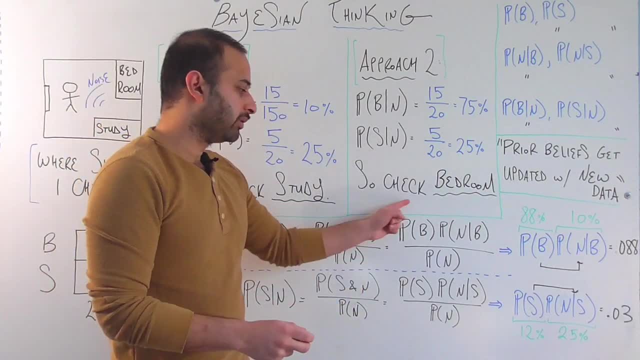 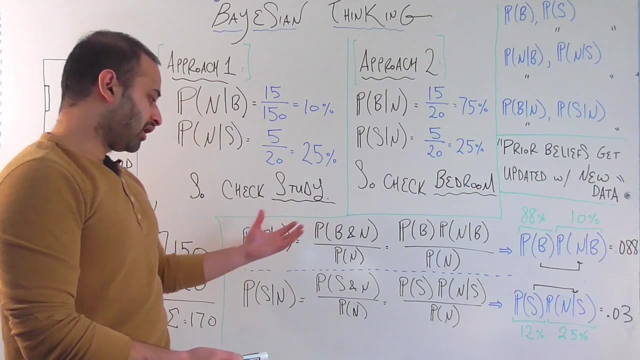 the way I've split it up here, Taking this numerator. split it up as probability of bedroom times, probability of noise given bedroom. So very important that you understand how I got from here to this form, This. yes, this is just called Bayes theorem, but I wanted to work it out from first. 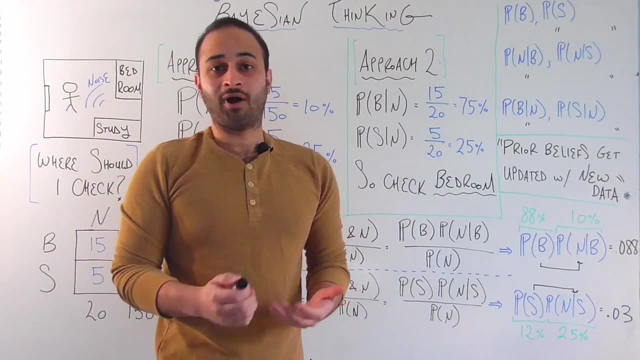 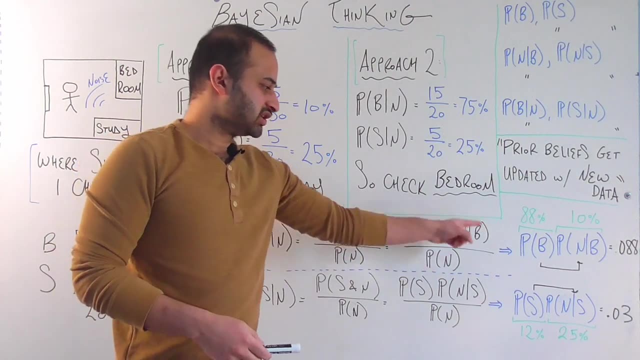 principles. in case anyone was unfamiliar or if you don't know why, Bayes theorem is true, And so we can work out the one on the bottom in a very similar way. So now we're just trying to figure out which of these is bigger. Is this quantity bigger or is this quantity bigger? Notice their. 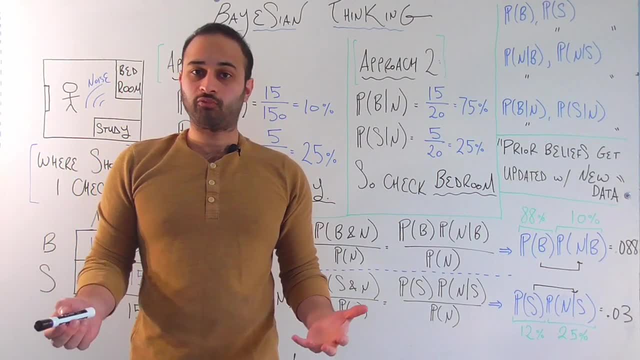 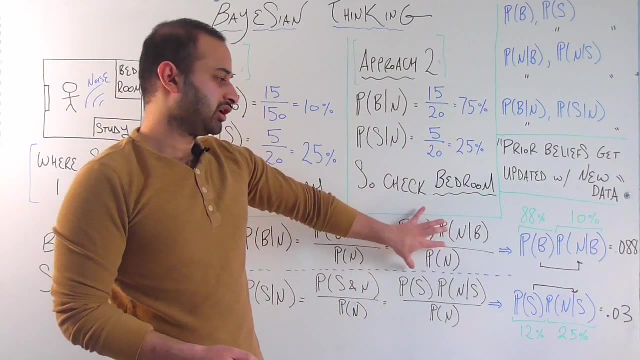 denominators are the same, so we don't even need to consider them. we just need to consider which numerator is bigger. So now we're kind of deciding between: is this quantity, which is the numerator here, is that bigger, or is this quantity, which is the numerator here, is that bigger? Before we 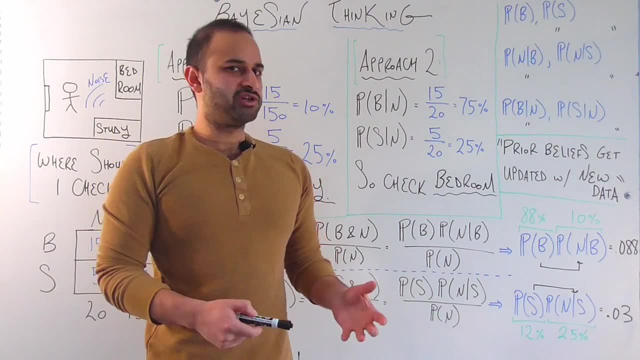 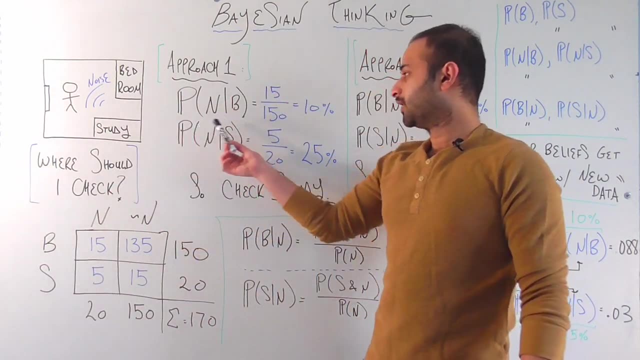 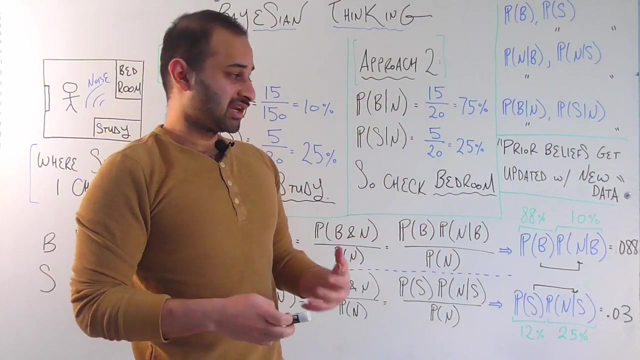 actually work out the numerical here. let's take a look at where. have we seen this quantities before? So probability of noise given bedroom. that was the quantity we computed right here, this 10%. So we see that, even though we are working in the context of approach two, we have started getting 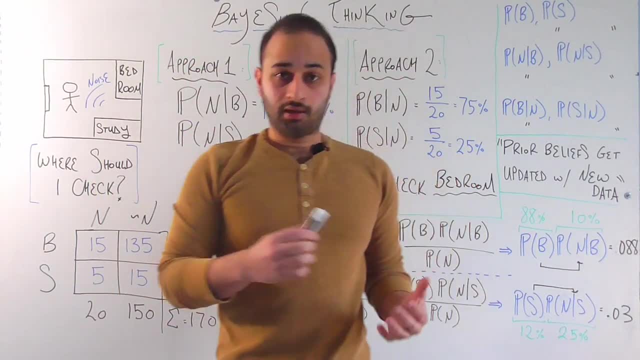 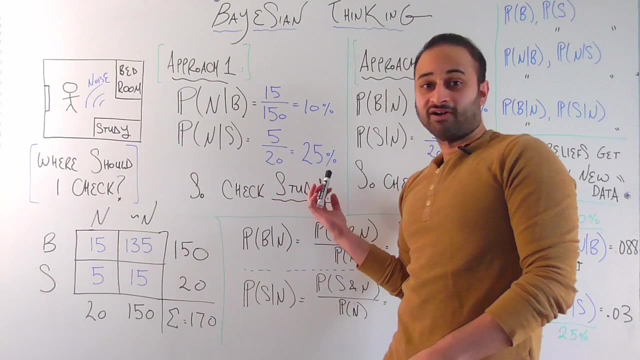 quantities that we got in the approach one, And we see that again by looking at probability of noise given study. that's the exact quantity we computed here: 25%. so now we start seeing the link between these. but that's not the only thing that are in. 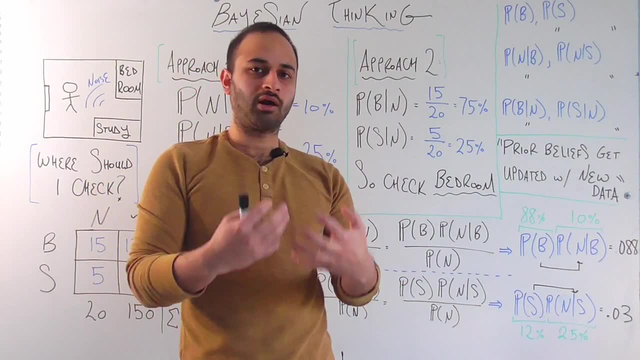 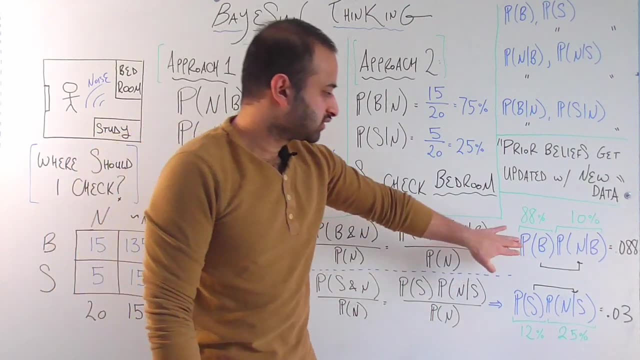 these formulas, there's two additional terms, and this is what leads to the heart of the difference between approach number one, which was not Bayesian, and approach number two, which is Bayesian. we get this first leading quantity here of probability of bedroom. let's think about what this means. this is saying that, not. 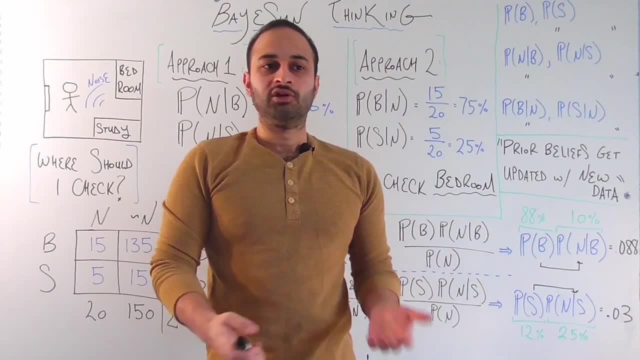 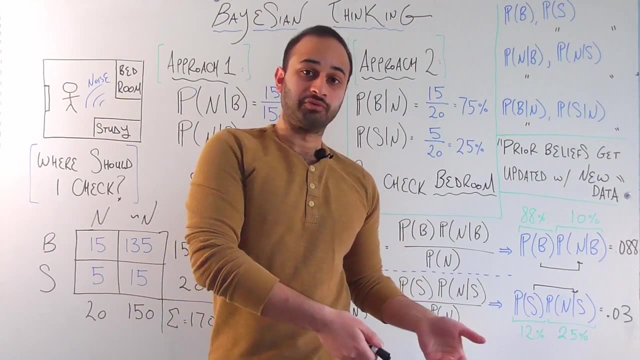 conditional on anything. I haven't even thought about the noise I'm hearing just if I walk in the door to my apartment. I don't even call the phone, yet what are the chances that it's in the bedroom? so this is kind of my prior belief. I'm 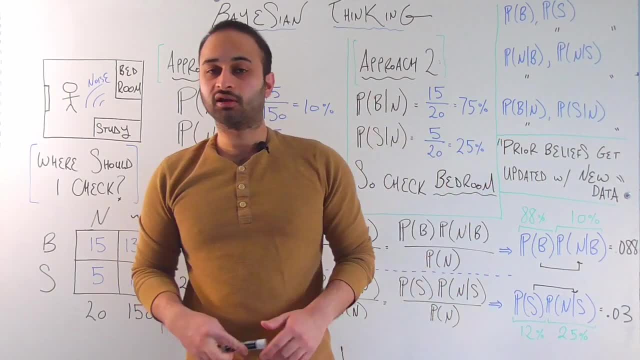 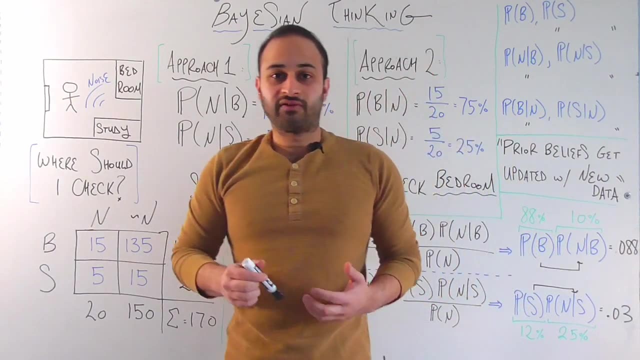 using that word prior very much on purpose, but we'll get to that in just a second. but this is my prior belief about where my phone is based on past data. this is saying that if I just walk in the door, I don't even call my cell phone. 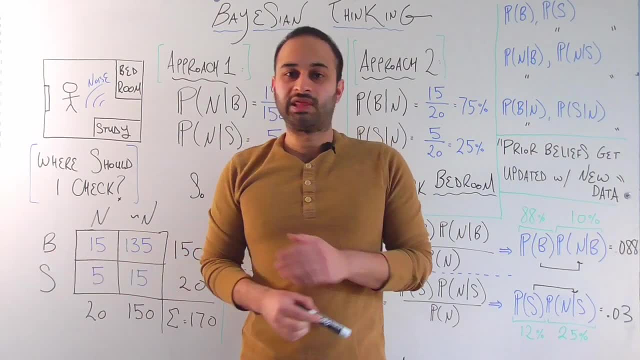 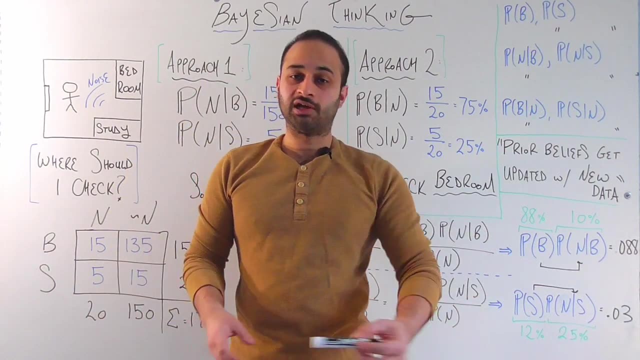 yet what is the probability? my phone is in the bedroom if I walk in the door, I don't even call my cell phone. yet what is the probability? my phone is in the bedroom without observing any data, and that's probability of B. similarly, what's the probability my phone is in the study as soon as I walk in the door? haven't? 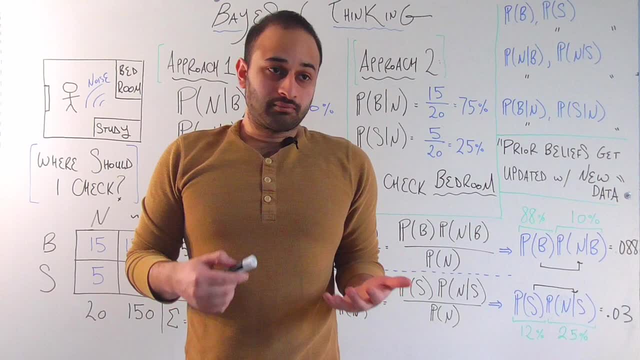 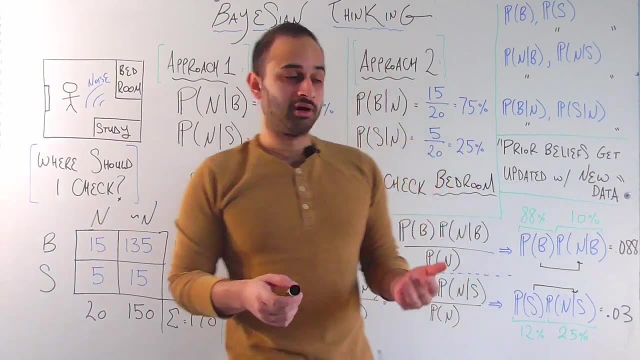 observed any data and that's probability of S, and we can actually get numbers for these right. what's the probability? my phone is in the bedroom. that happens a hundred and fifty times out of 170, so that's about 88 percent. what's the probability my phone is in the study? that has to just be the complement of 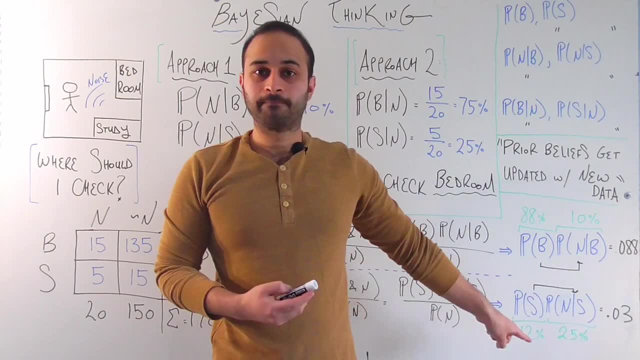 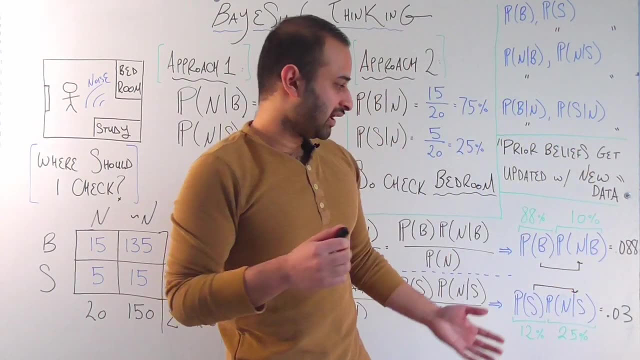 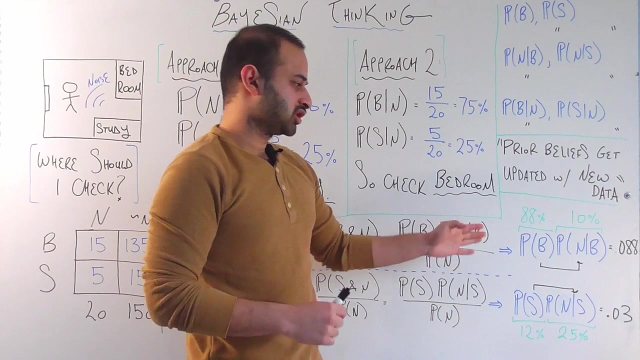 that because they add up to one and that's twelve percent. if I multiply those by these two numbers, which again comes straight from approach number one, then I get point zero eight eight on the top and point zero three on the bottom, and that explains numerically again why I chose to go with. 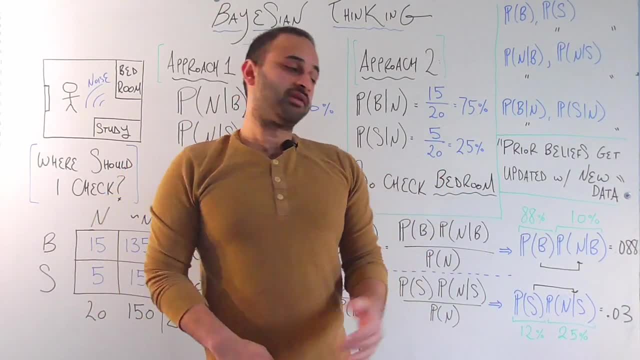 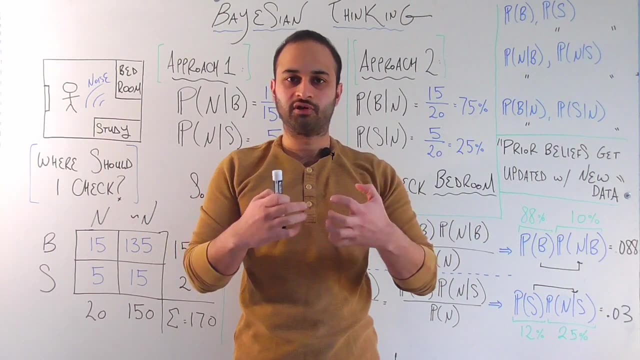 the bedroom in this case, because point zero eight eight is higher than point zero three. but let's try to frame this further in terms of a story, because we're almost there. all the parts are here, we just need to link them together into a narrative. what does approach number two add on top of approach number? 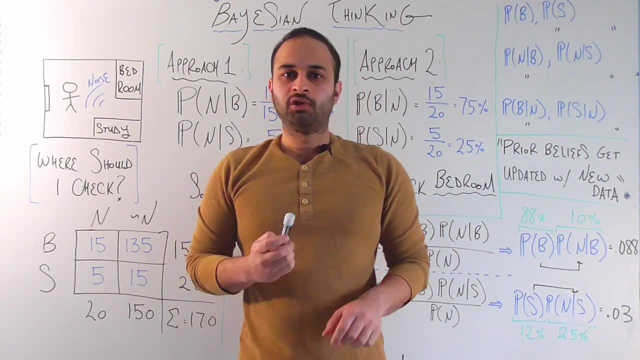 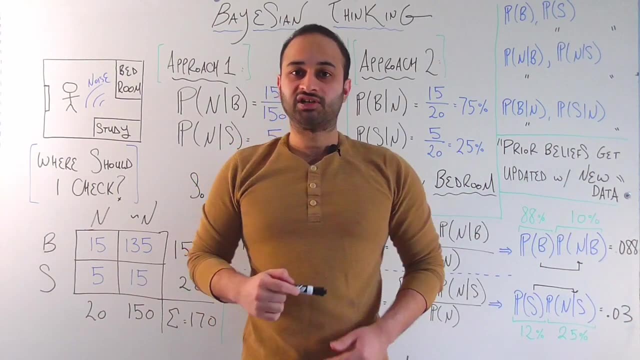 one. so let's look at this top one here. this is saying that I walk in the door and I haven't even called my phone, and I know that there's a 88% chance that my phone is in the bedroom and a 12% chance that my phone is in the study. so if I 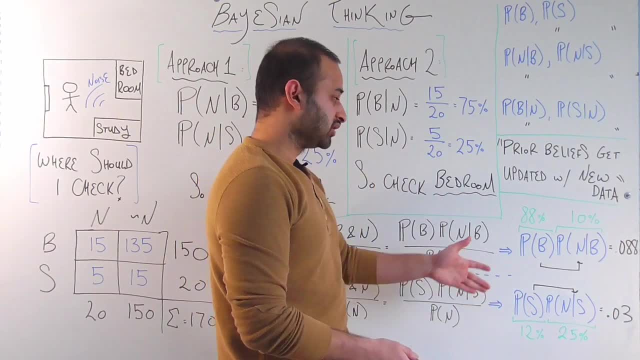 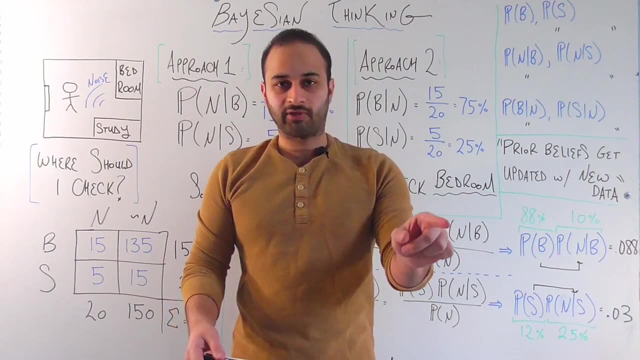 were to stop here, at just these prior beliefs, I would go ahead and check the bedroom for sure. by far, 88% is much bigger than 12%. but I don't stop there. I observe some data about the world. I observe some data about the world. I. 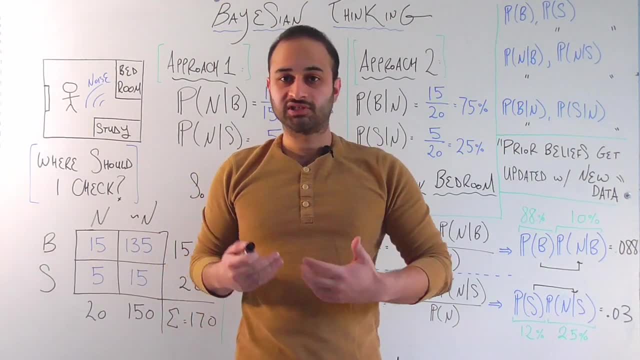 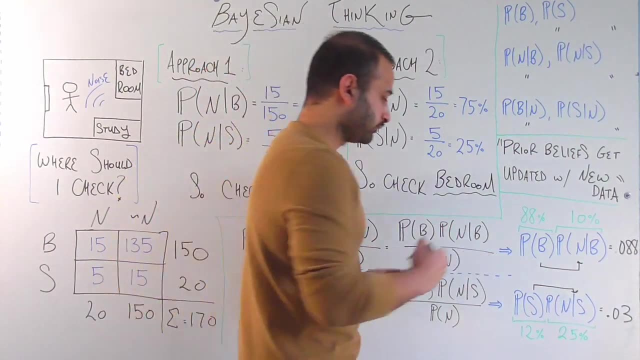 which is that I call my phone and I observe the noise. I hear the noise that comes back. the purpose that that serves is to update these prior beliefs, so that's what I'm gonna write here. so the sense in which we update the prior beliefs is that we say, okay, now I call my phone. now, given that my phone was in. 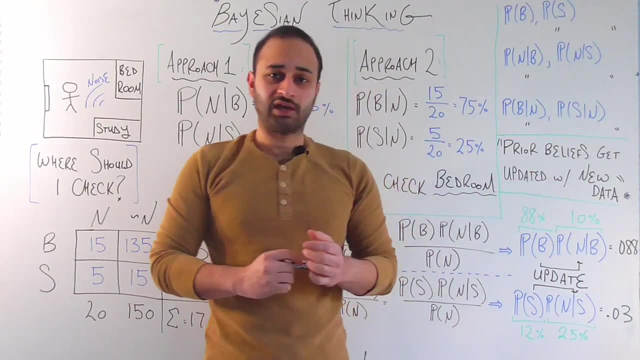 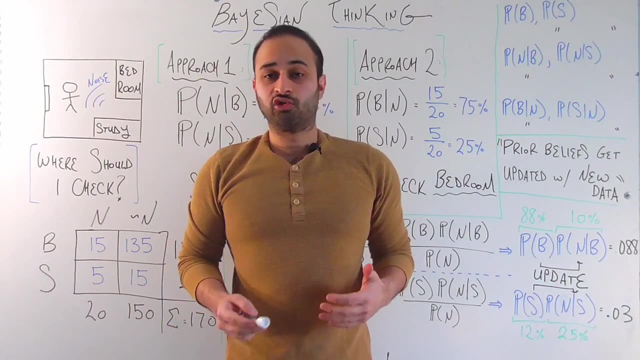 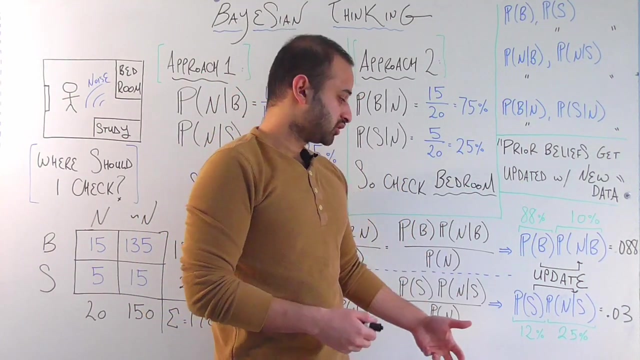 the bedroom, the probability of hearing that noise would be only 10%. so, even though there's a very high chance of my phone being in the bedroom before hearing the noise, hearing this noise causes us to apply this 10% factor on to this 88% prior. what does it do to our other situation? so, even though there's 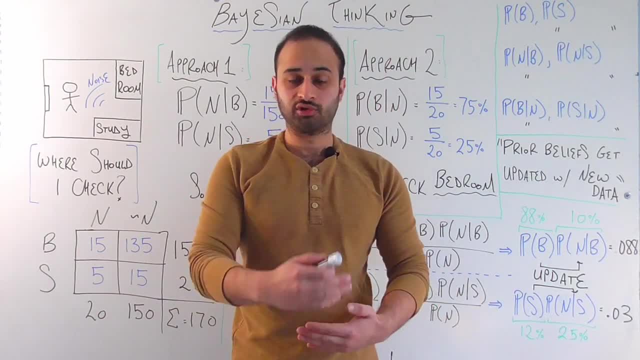 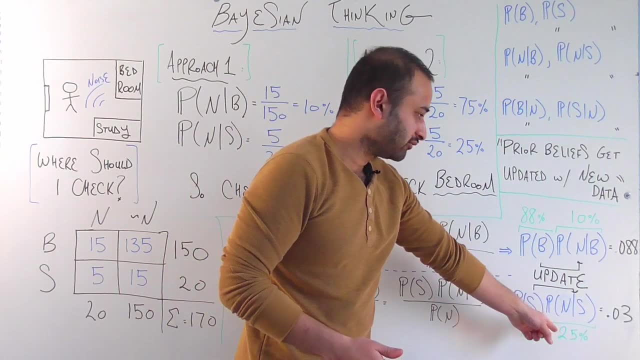 only a 12% chance that my phone is in the study. as soon as I walk in before I call the phone or anything after I call the phone, I go ahead and update those beliefs by multiplying this factor of 0.25 and notice this is telling the full. 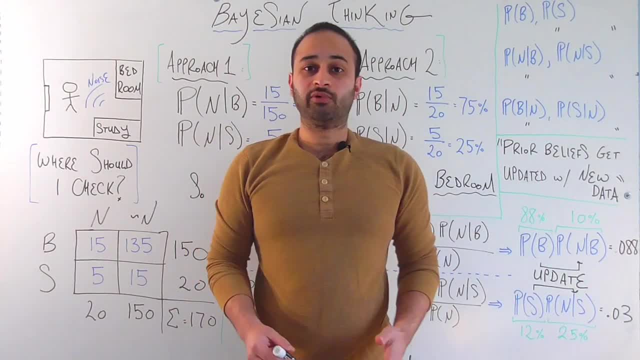 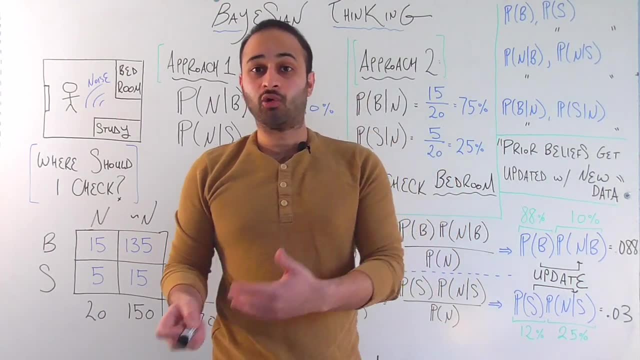 story because 0.25 is bigger than 0.1. so even though to begin with there's only a 12% chance of my phone being in the study, we're saying that under the assumption of the phone is in the study, probability that I would hear that noise. 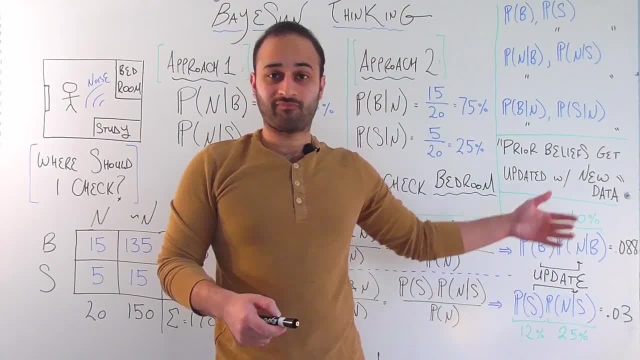 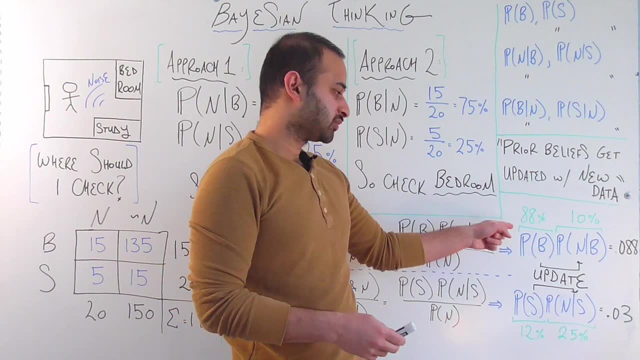 actually much higher than the probability of hearing the noise if my phone was in the bedroom. so another way to think about it is that I am decreasing this prior by a smaller amount, that I am decreasing this prior. so, even though this was 88%, I'm only taking 10% of that going forward versus 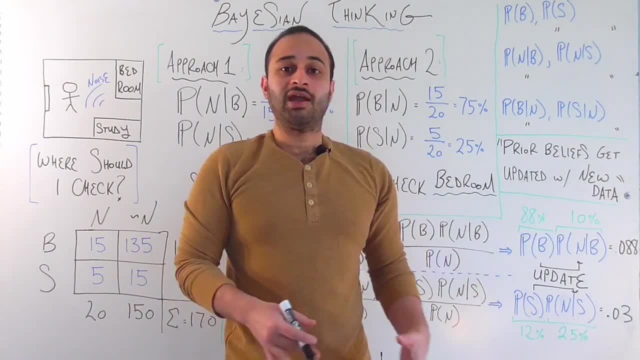 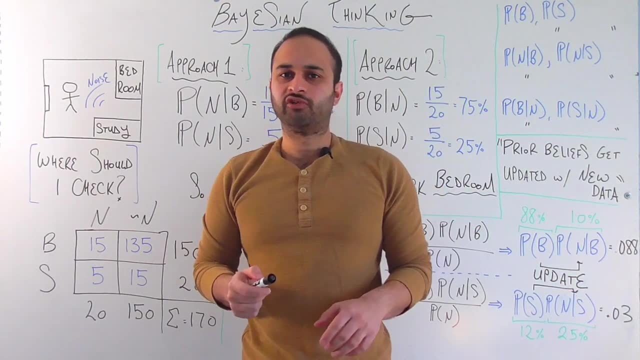 this was 12%, but I'm taking a whole 25% of it going forward and the conclusion we get is that we should still check the bedroom, but notice that 0.088 and 0.03 are only a magnitude of about three apart, so about triple. 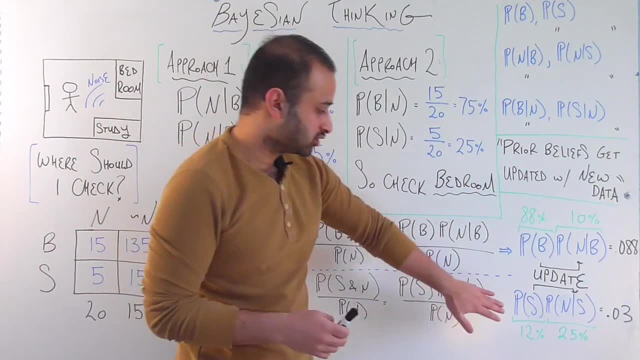 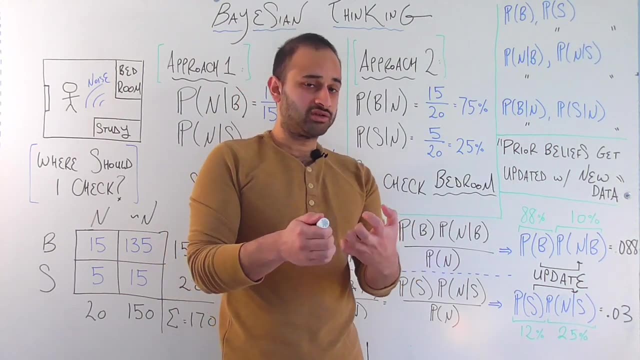 but if we didn't observe the data at all, the magnitude of difference between 12% and 88% is about a factor of seven. so even though the conclusion didn't change, we got a lot closer to thinking that the phone was in the study, and now we truly. 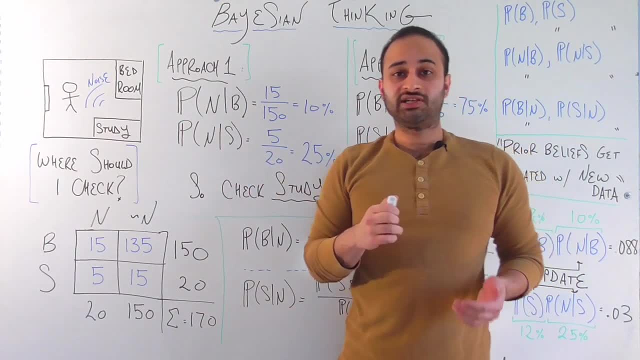 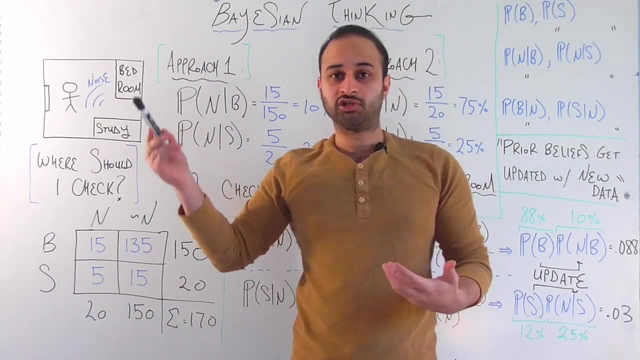 learned the difference between these two methods. approach number one does not take into account at all the pure probability or the prior probability that the phone was in either of these rooms. it treats those as equal, and that may or may not be a good assumption. in this case, we see, it's not a good. 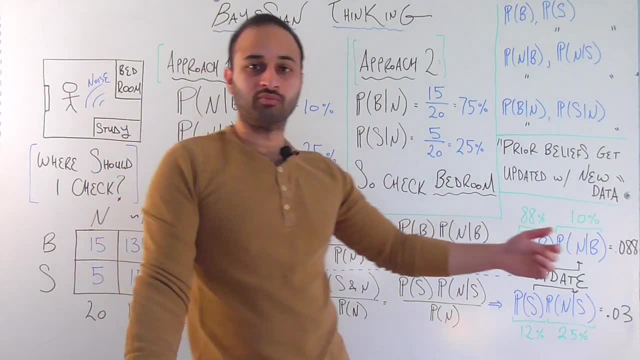 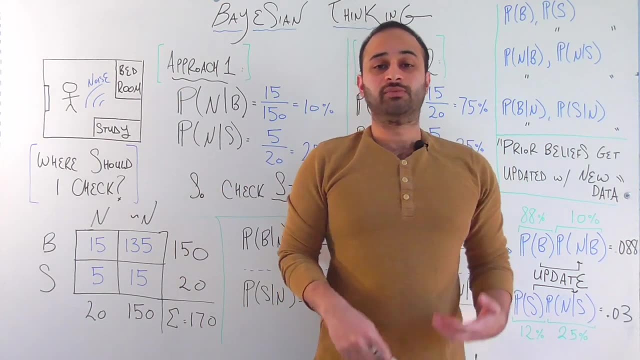 assumption there's a much higher chance prior the phone would be in the bedroom than the study. but in some situations maybe it is a good assumption, in which case both of these approaches arrive at the same exact answer. so approach number two in a sense builds upon approach number one by considering actually what 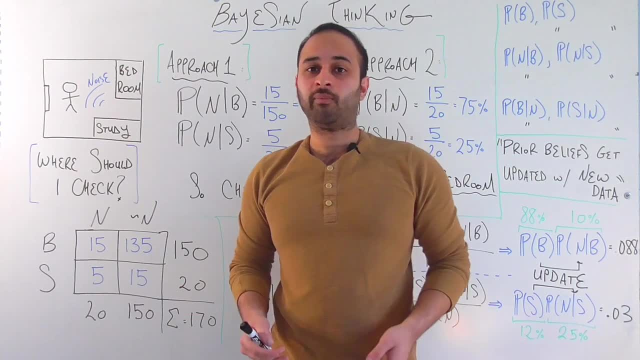 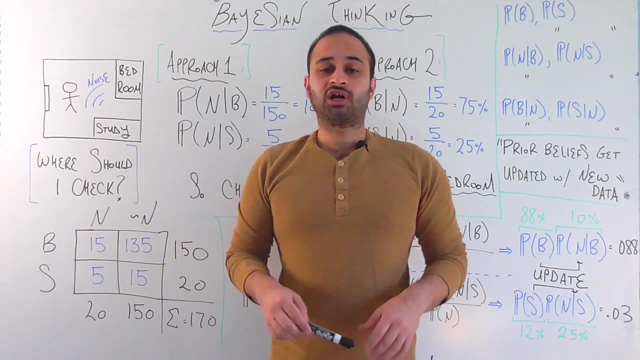 is the prior probability of this event, and then updates that prior probability after learning about new data. so let me give a couple of labels to all the probabilities that we've been talking about, and then we'll talk about the pros and cons of Bayesian reasoning. so, probability of B, probability of S, as I've 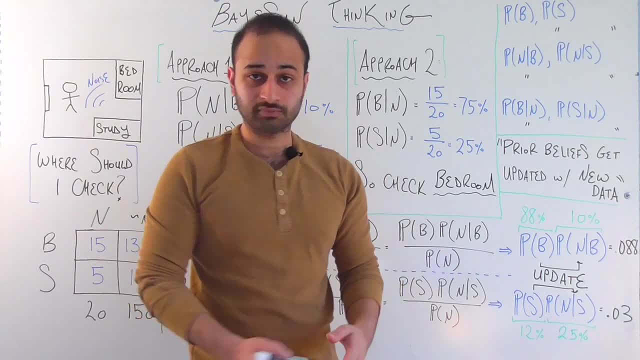 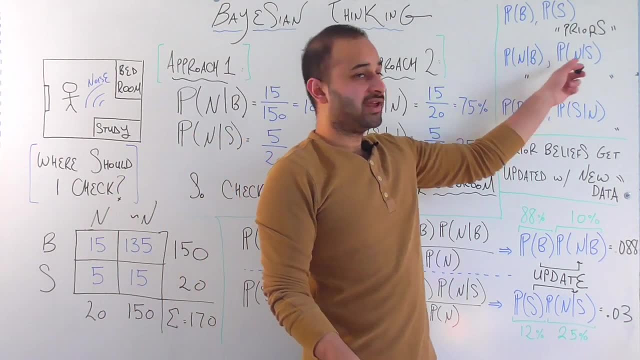 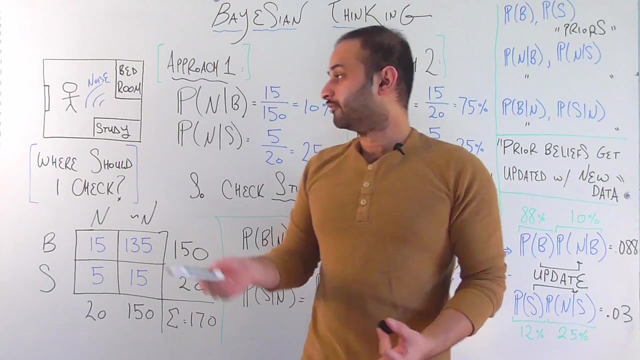 been calling them this whole time, are called prior probabilities or just priors. so this is our assumption about the world before learning any data. probability of N given B and probability of N given S, which were the first ones we computed over here, are called likelihoods. so this is saying that what is the likelihood of seeing? 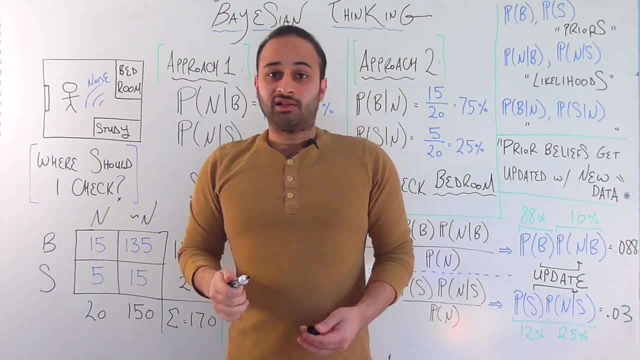 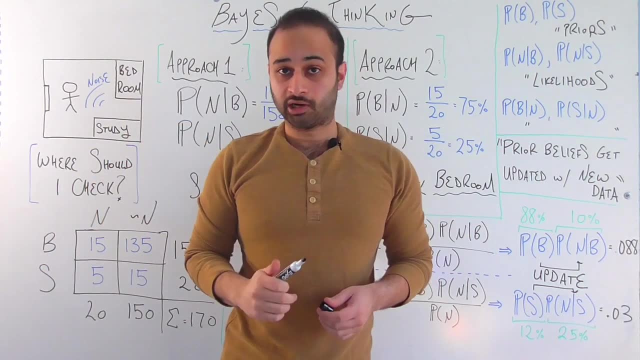 this data in the real world, if this unknown thing is true. and finally, the probability we computed in approach number two, which was probability of B given N and probability of S given N, are called posteriors, which means that, given that I have my prior after, I incorporate information about the real 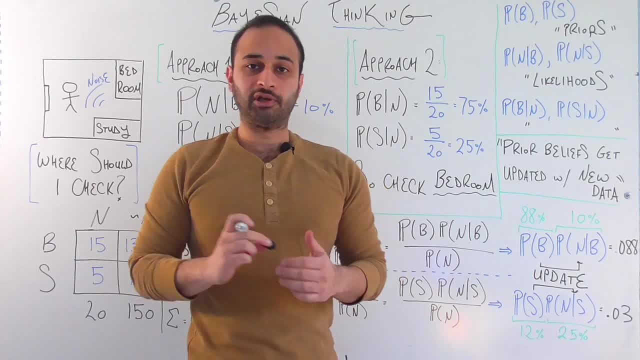 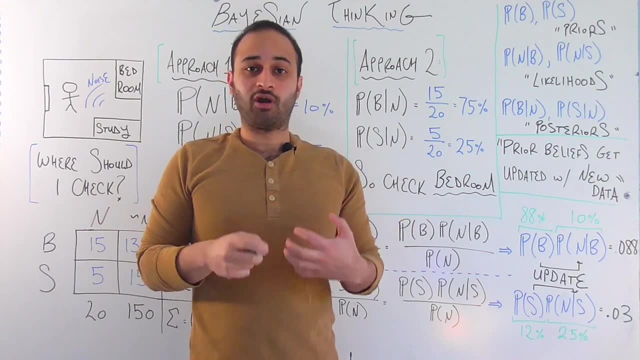 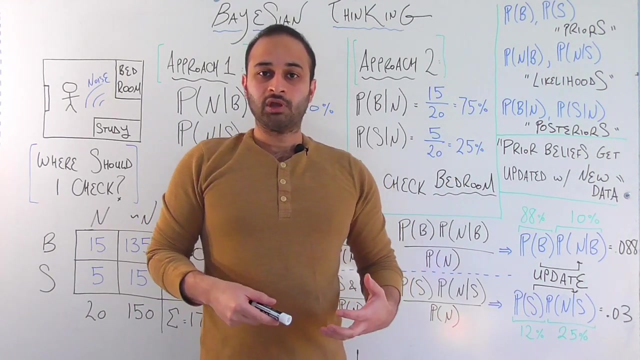 world, which is likelihoods. this is my posterior probability, and so, again, I just want to hit this point home. make sure it's not unclear in any way. the heart of Bayesian reasoning, if I had to sum it up in one phrase, is that prior beliefs about the world get updated as we learn new data. so we have some. 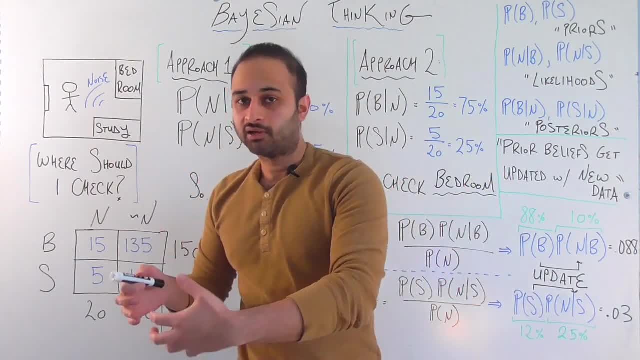 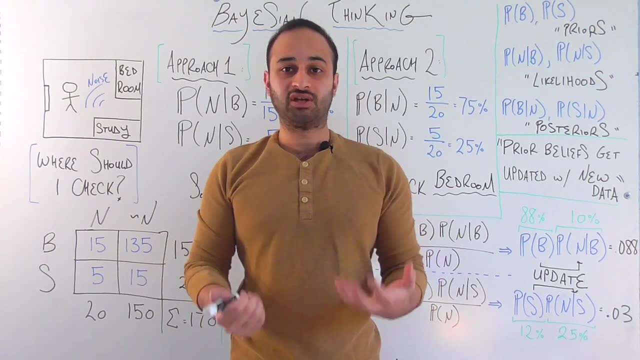 initial understanding of the world. we learn data, we learn data, we learn data, and then we update these beliefs accordingly, and personally, I think this is. the biggest problem in the world is that we don't know exactly what is the pro of Bayesian thinking, because this is how human beings reason about the world anyways. 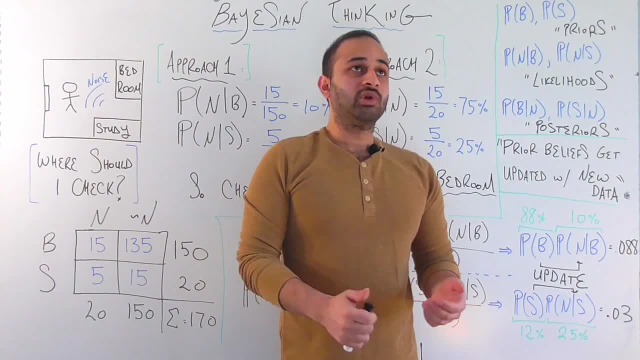 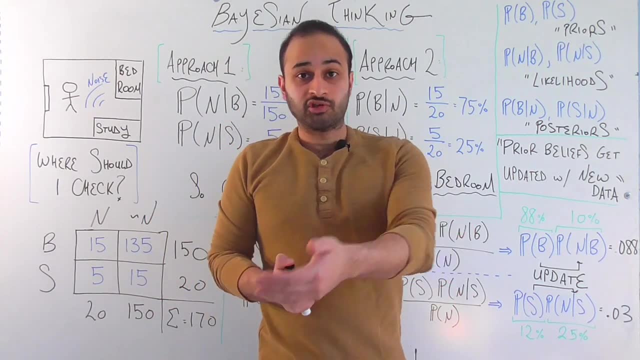 for example, let's take a situation of looking for a job. before you even go to the interview for the job, you have some kind of prior belief that I'll get the job. maybe it's like 50%. then you go to the job, you go to the interview and you get some kind of positive feedback. 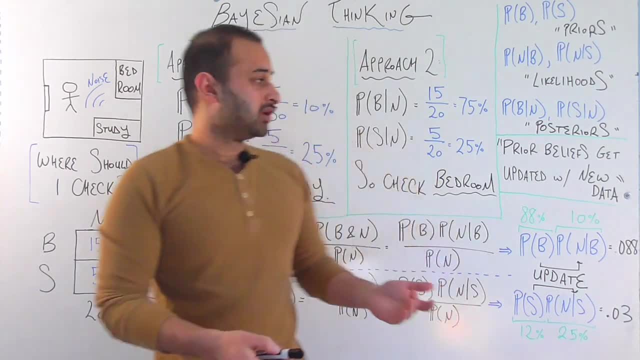 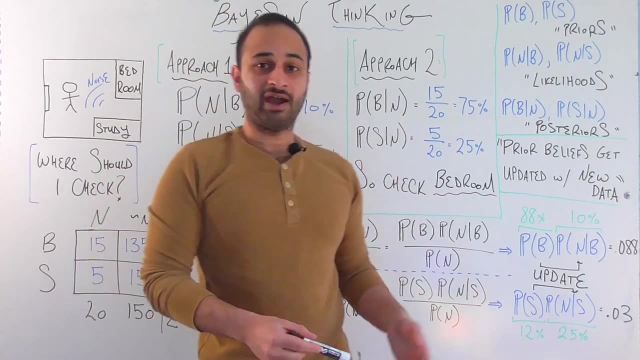 from your interviewer. that is going to change that prior belief. now the probability of job given positive feedback again, job is still unknown whether you got it or not, but the positive feedback is data based on the prior belief. so we know that it's a positive feedback for the job and we can let it go and we can add more information on it later on, but it's 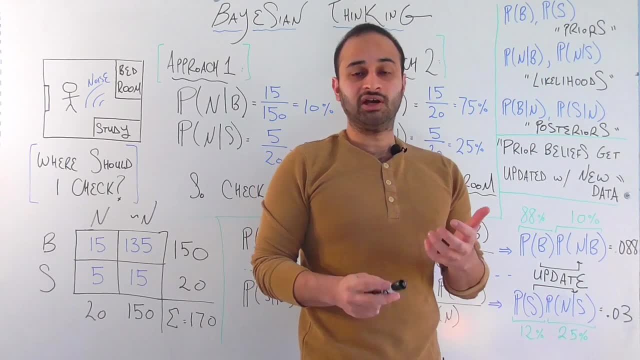 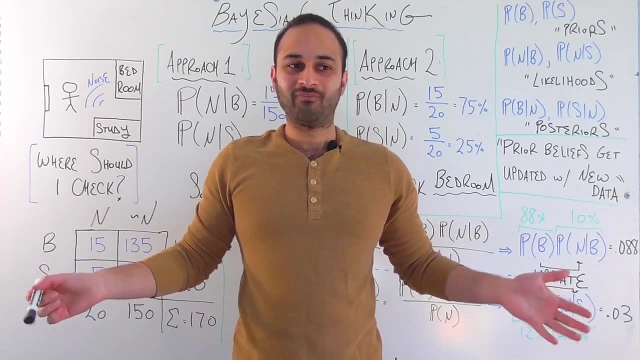 that you did observe. that probably goes up. maybe now your probability of thinking you got the job given the positive feedback is 75. then let's say you wait a week and don't hear anything back at all. now you adjust your beliefs again now probability of job given positive feedback. 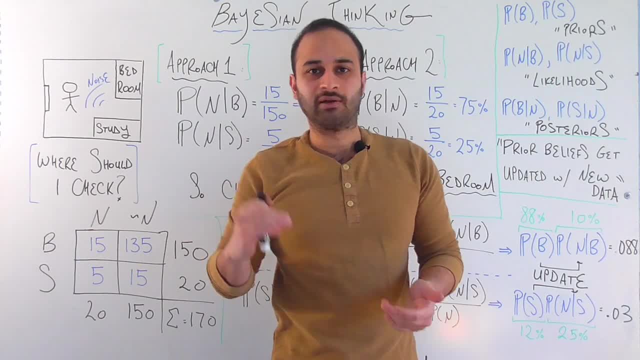 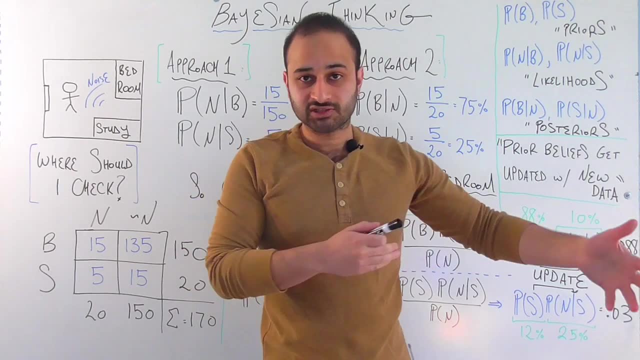 but you haven't heard back for a week. maybe that's down to 60. so this is how we think about the world. we kind of have an assumption about what's the probability of something happening, but then as we observe events, as we observe data, we kind of update that in our minds. so i think that's the 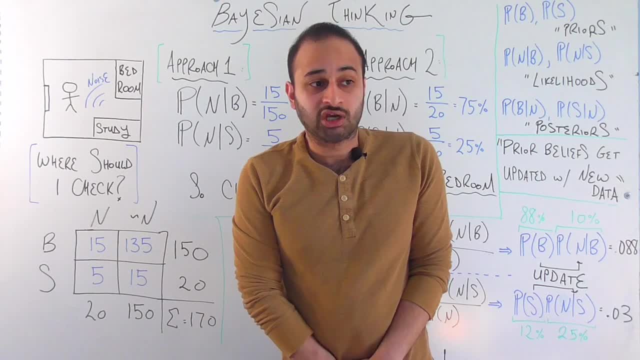 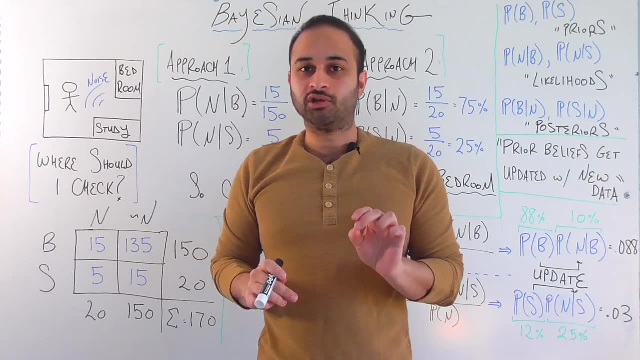 biggest pro of bayesian thinking. now let's finish this video by talking about the biggest con of bayesian reasoning, which i've kind of been glancing over, and that biggest con is exactly how you construct these prior beliefs. so think about these probabilities. which ones are the easiest to get? 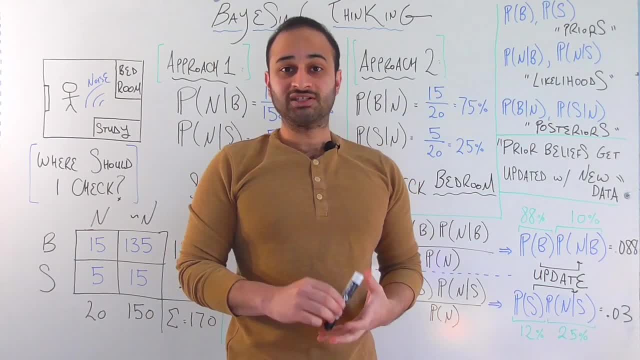 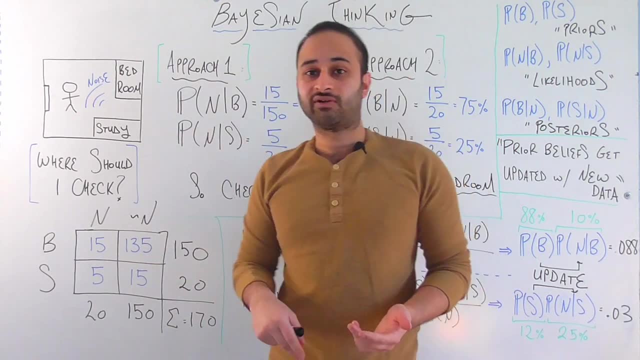 looking at the likelihoods, this is the probability of hearing the noise. given i left the phone in a certain room, i can actually just do a simulation. you can actually just do a simulation and you can actually just do a simulation and you can in one evening. i can just leave the phone in the bedroom in several places. i can leave the room in. 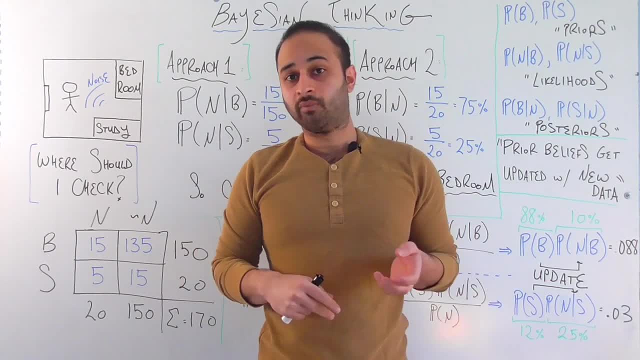 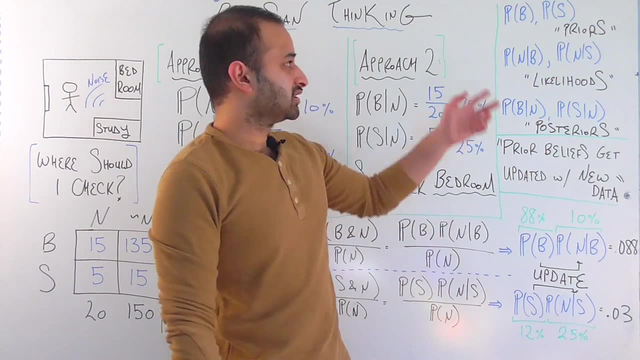 the study in several places and then call it and observe what's the probability of hearing the noise. pretty easy to do. i could just take an afternoon or an evening and do that. what's harder to get is the priors, which is the probability that i do leave my phone in the bedroom or i do.